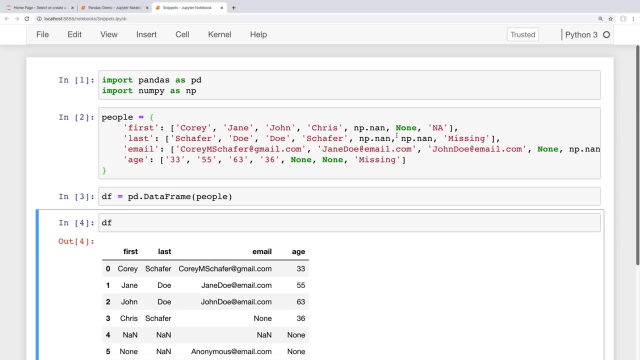 videos we'll learn how to do some of this in our smaller snippets data frame first, And then we'll see how to do some interesting stuff on our larger Stack Overflow data set to get this working on some real world data. So for this video I've added some null values here into our snippets. 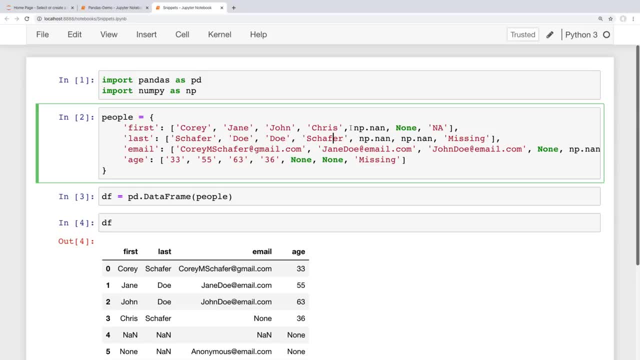 data frame that we didn't have before. So I added some extra first names here And we can see that I just have one that is a numpynan, which is a, not a number value. I also imported numpy up here at the top. This and this one here is just a none value. And then I also have some custom missing. 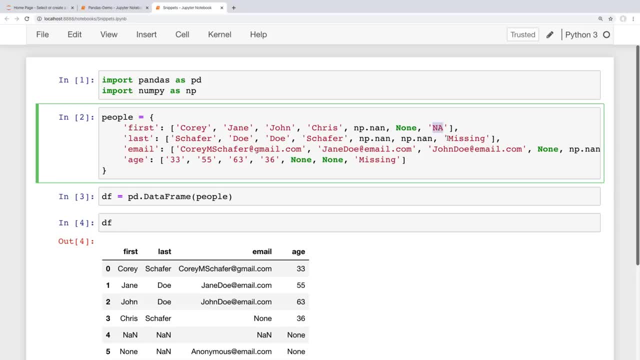 values as well. This one is just a string of na And this one is just a string of missing, So I don't have any of that thrown throughout this data so that we have some missing values. So you're going to see this a lot, that when we work with pandas we're going to have some missing data And 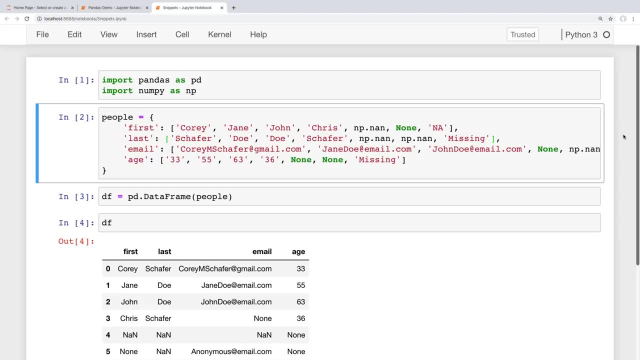 depending on what it is you're trying to do, you might want to handle this in different ways. So one thing you might want to do with missing data is to simply remove it. So for our small data frame here, let's say that we're going to do some analysis with these people in the data frame. But 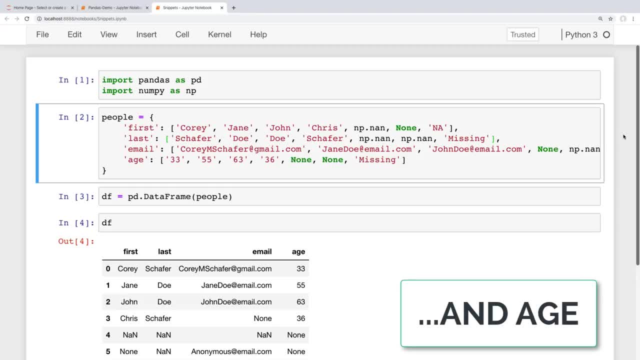 if they don't have their first name, last name and email address, then we can't do what we want to do with them. So we're going to go ahead and do that. And then we're going to go ahead and do some analysis with them. And then we're going to go ahead and do some analysis with them. So we'll. 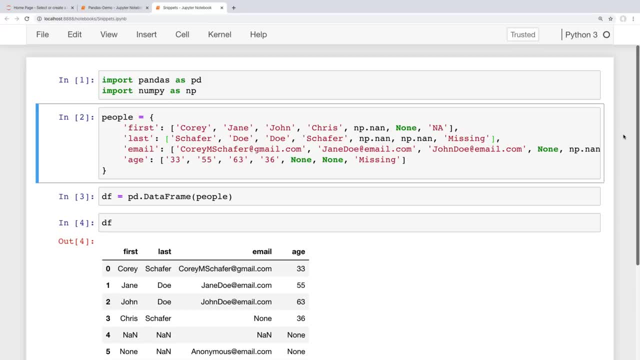 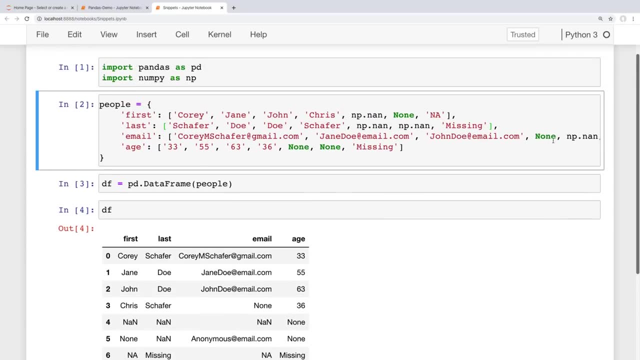 just remove the rows that don't have those values. So in order to do this, we can use the drop in a method. So let's do this And then I'll explain the results and go over those. So all I'm going to do down here with my data frame is I'm going to say df, dot, drop in a, and we're going to run. 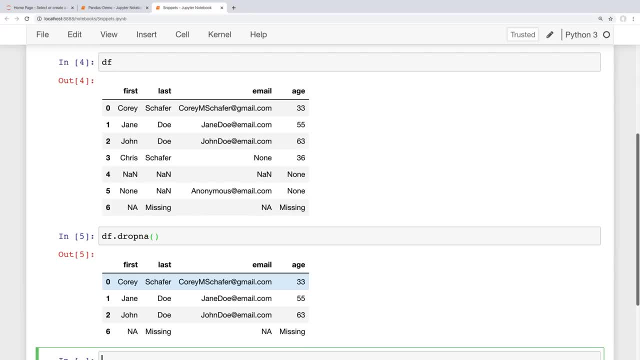 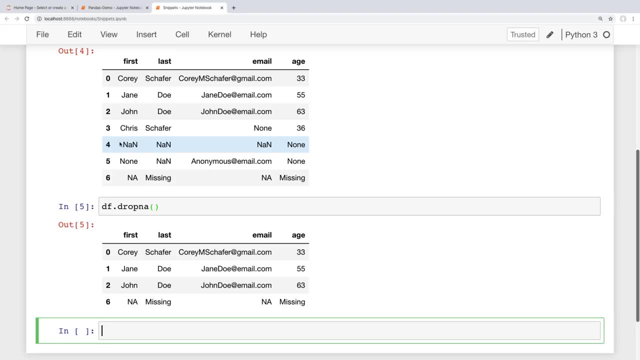 that without any arguments right now. So when we run this, we can see that now we only get four rows of data here, And up here we had, let's see, four, five, six, seven. so we got these four rows here because they didn't have any missing values. Now we do still. 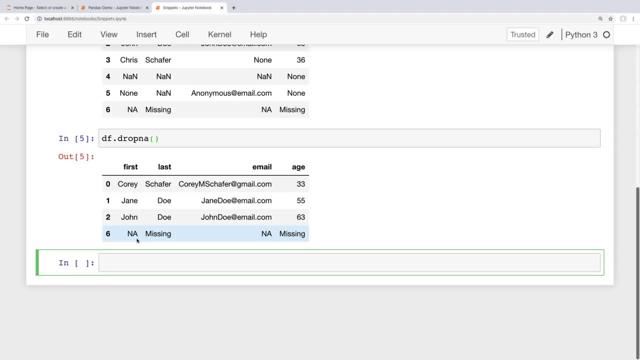 have our bottom row here, which has some of our custom missing values, But we'll see how to deal with these in just a second, But for now, let's go over what drop in a is actually doing here. Now, what's going on in the background is that drop in a is using some default arguments, So I'm going 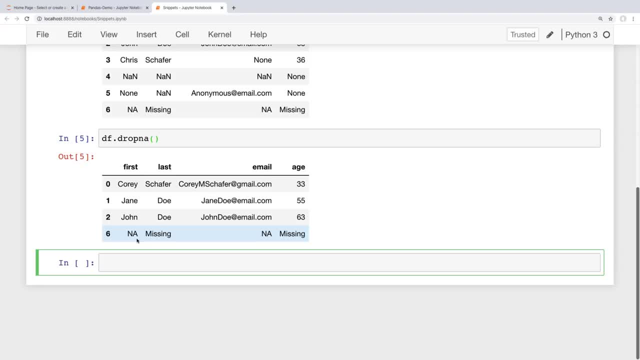 to manually fill in these default arguments And it might make more sense why we got this specific result. So, by default, we're going to have a default argument And we're going to have a default argument. And we're going to have a default argument And we're going to have a default argument. 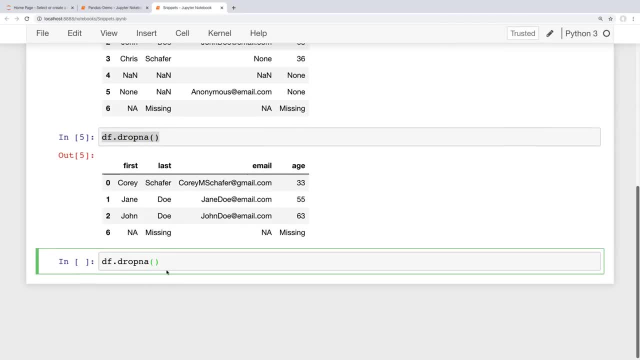 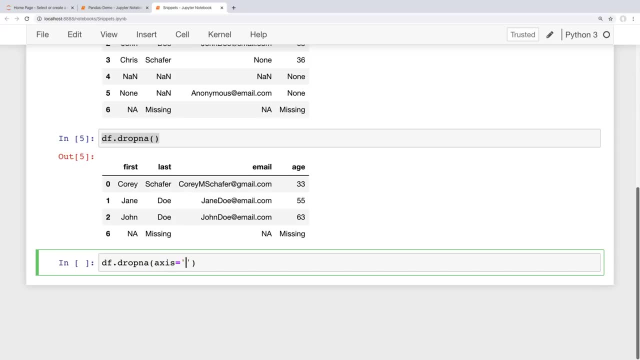 By default. I'll leave that one here, And now I'm going to fill in, drop in a again, but I'm going to put the default arguments that it already has, And the default arguments of what this is doing in the background is it has an axis set to index and it has a how variable set to any. So, since 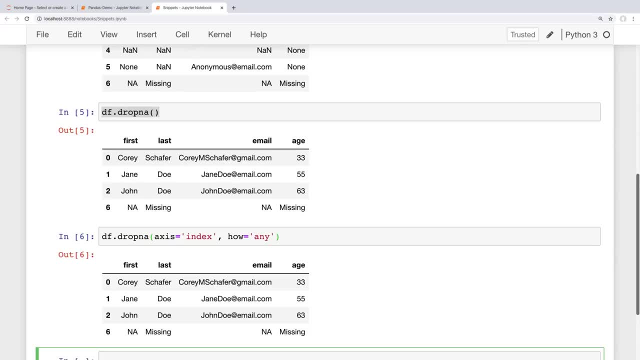 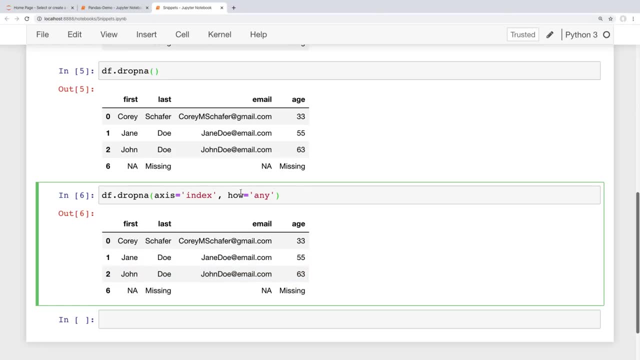 this is what the method was using by default. anyway. we should go ahead and get the same results here, And we can see that we do. we get the same results as we did when we ran this up here. But now let me actually explain these arguments here. So first we have the axis argument, So this: 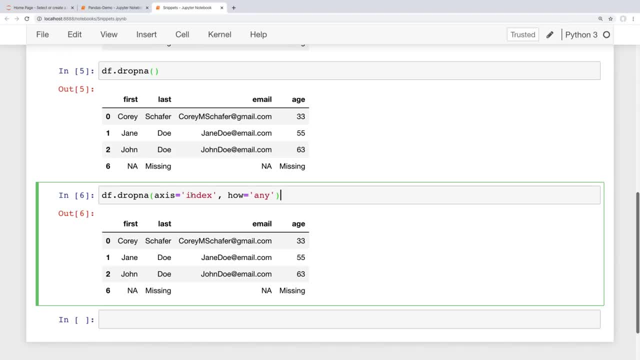 can either be set to index or set to columns. that is going to tell pandas that we want to drop in a values when our rows are missing values when it's set here to index. If we set this to columns, then it would instead drop columns if they had missing values And we'll look at that in just a. 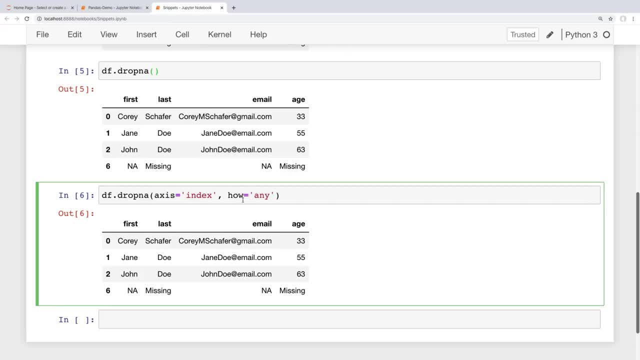 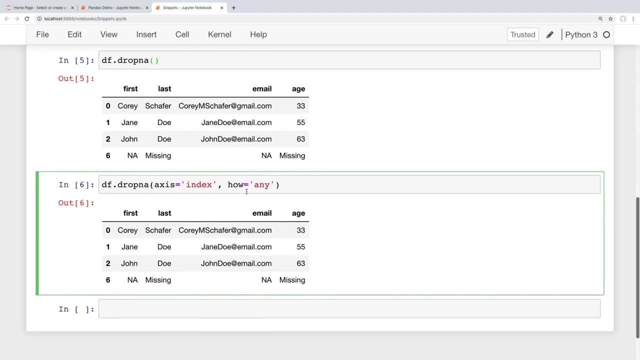 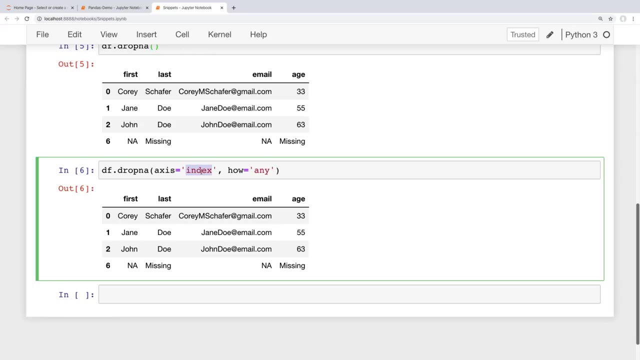 second. Now the second argument here is how we want to drop these, or I guess a better way to frame that is: this is the criteria that it uses for dropping a row or a column. So by default, this is set to any. So we're looking over our rows, since this is set to index and this is set. 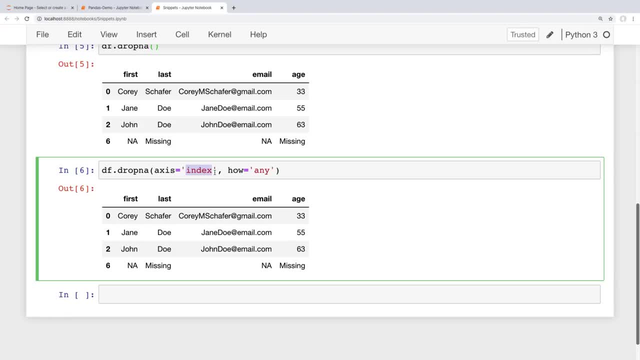 to any here, So it will drop rows with any missing values. But this might not be what you want, Maybe with this kind of an analysis that we're doing. it's okay to have you know missing email or last name or something like that, But there just has to be something that we want to drop in here. 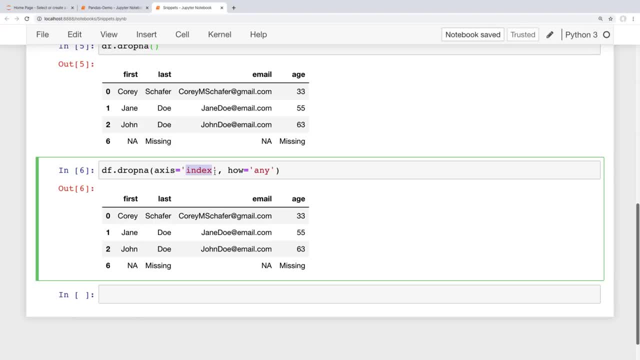 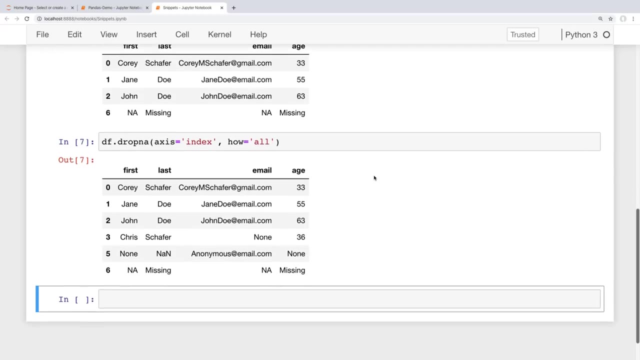 Something. it can't just be an entire row of missing values. So if that's the case, then we can instead change this how argument to all, And this will then only drop rows when all of the values in that row are missing. So now, if I run this, then we can see that now we get back more rows than we. 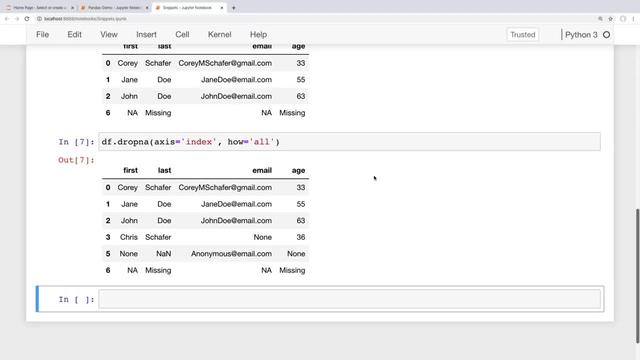 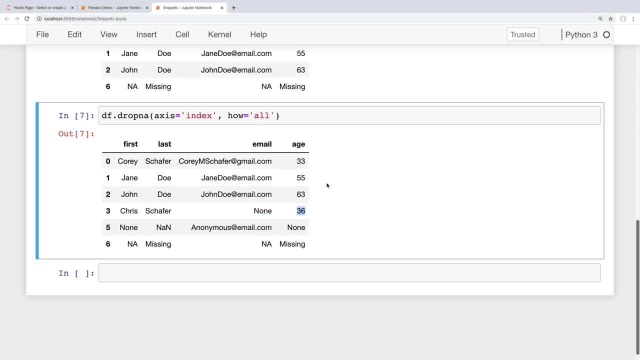 did before, because it kept the rows that had some missing values, but not all missing values. So we can see here we have an email missing, but there were some other columns filled in And we can see that everything was missing here, But they did have. 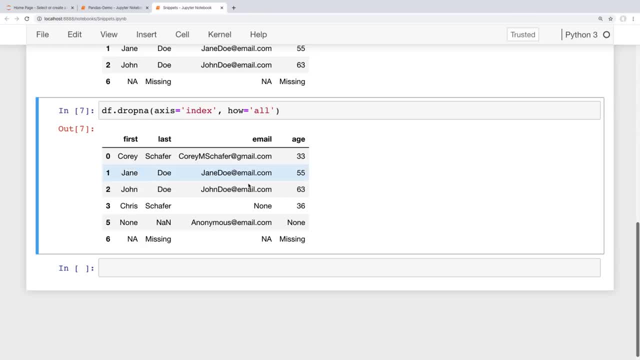 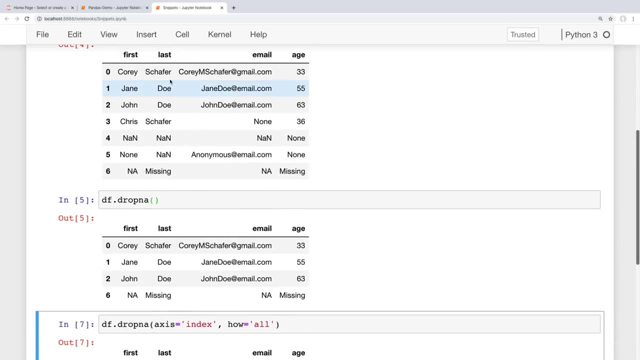 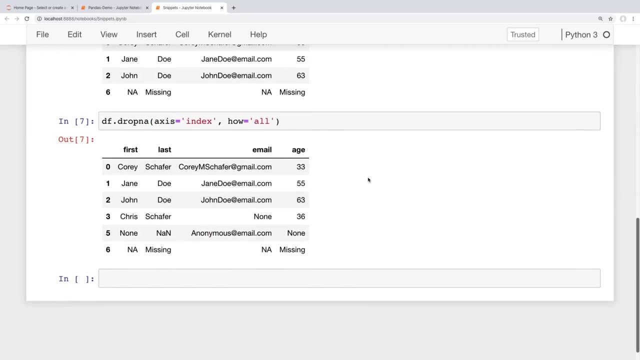 an email. So all of the values have to be missing in order for this to actually drop those. So it looks like we are missing index of four. If I go up to my original data frame here, we can see that that index had all missing values there. Okay, now, if I instead change this, access to columns. 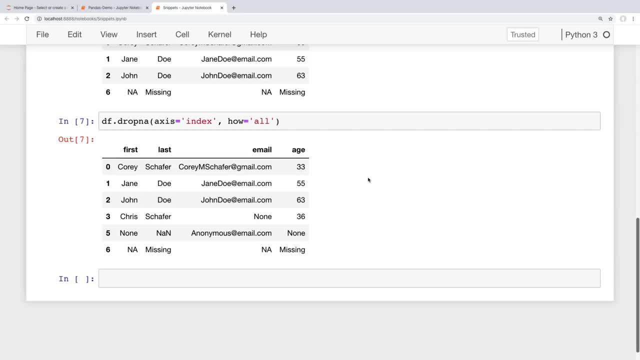 instead of index, then it will drop columns that have all missing values. We don't have any columns that have missing values all the way down, So it should just return our original data frame. So if I say columns here and run this, then we can see that that's what we get, Because none of these columns 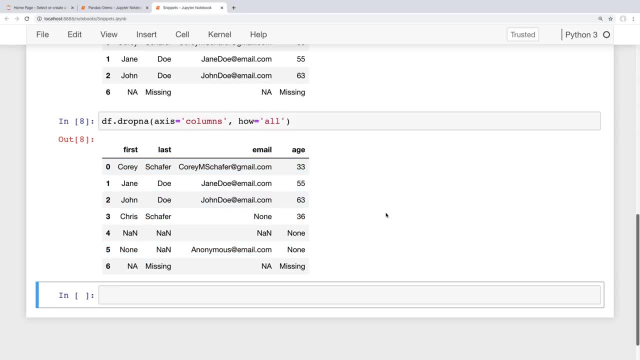 have missing values all the way down. Now, if I set this back to the default and drop columns with any missing values, then we'll actually get an empty data frame returned, Because we have one row that is completely empty, that we saw here, this index of four. So for that row, 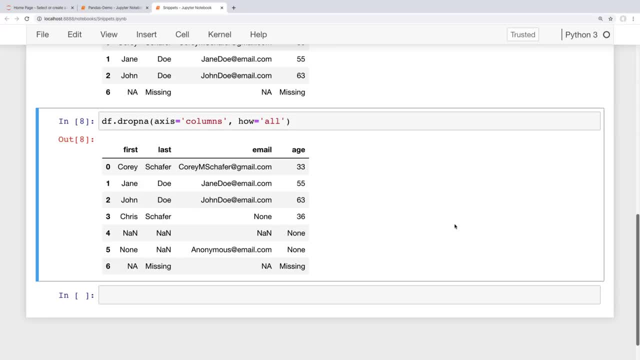 each column is going to have at least one missing value, And if we set this to any, then any column which is even a single missing value will be dropped, which in this case is all of them. So if I change this to any, then, since we have all missing values in one of these rows, 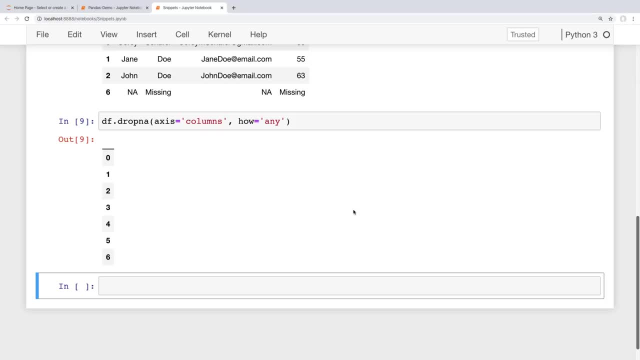 that's just going to give us an empty data frame. Now, at this point, you might be wondering: okay, well, my data is a bit more complicated than this and I'm doing some analysis where I want to drop some missing values, but I only want to drop rows. 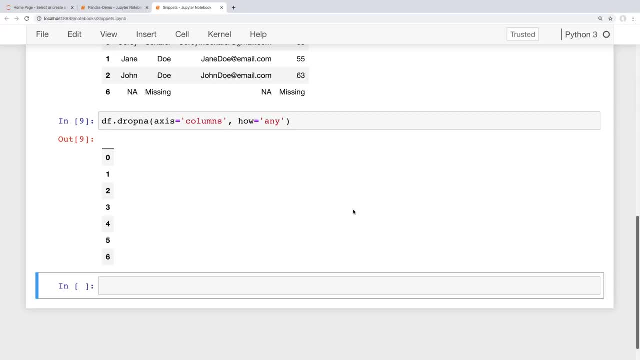 that are missing values in a specific column. So, for example, let's say that we're doing some analysis on our data and it's fine if they don't have a first name or a last name, but we really need the email address. And if they don't have an email address, then we need to just drop those. 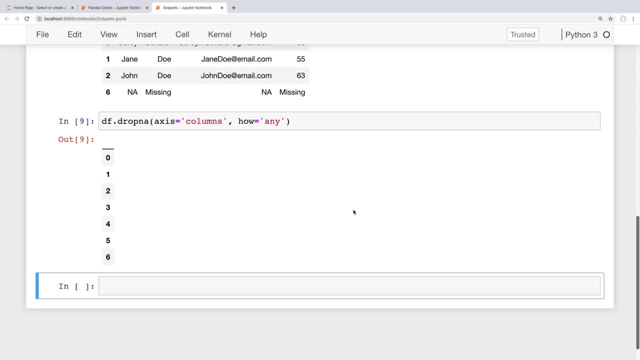 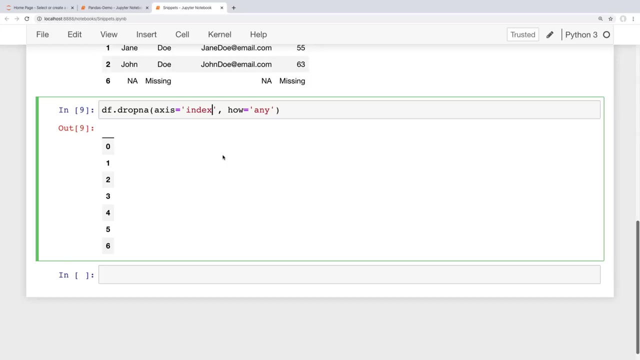 rows. So in order to do this, we can pass in a subset argument. So first I'm going to set our access here back to index so that we're dropping rows, And now we want to pass in a subset argument, And this subset will be the column names that we're checking for missing values. So in this, 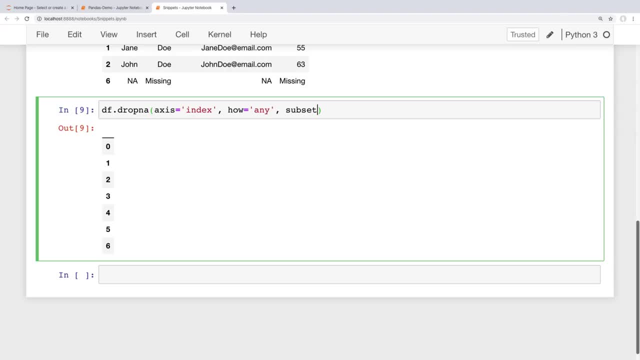 case it's just going to be a single column. So I'm going to say: subset is equal to, and I'm still going to pass in a list, even though this is just a single column, and I'll say email. So if I run, 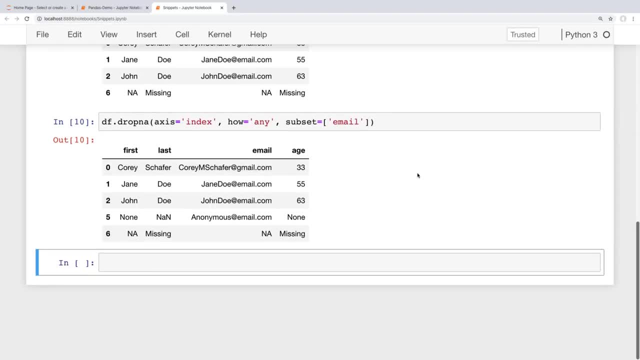 this. then we can see that the data frame that we get back is going to be a single column. So we're going to say that the data frame that we get back is full of rows that have at least their email address filled in, And again this one down here with these NA values. that is our custom. 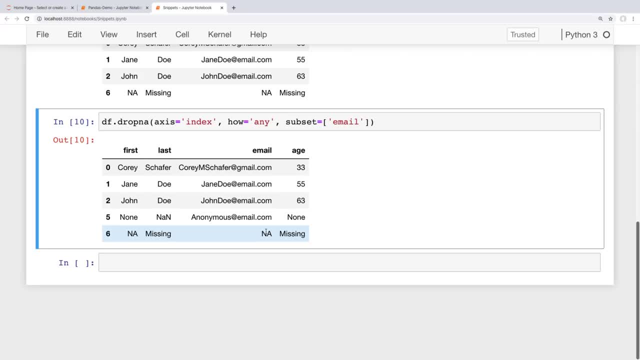 missing values, And I'll show you how to treat those as missing values in just a bit Now. in this case here, since we're only passing in a single column for our subset, our how argument here isn't really doing much, because it's only going to look at the email address for missing. 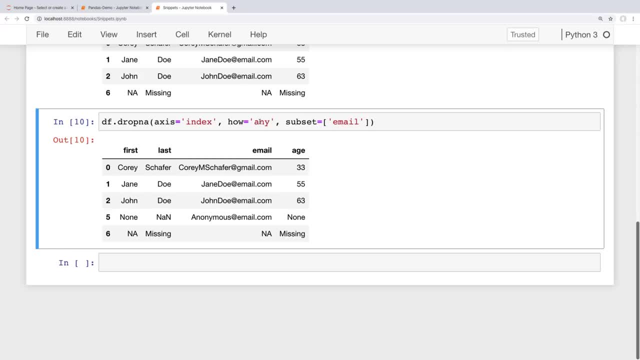 values. So if an email address isn't filled in, then passing in either any or all for the argument here would trigger that row to be removed. So even if I put this as all, it should give us the same results, because we're only checking one value, But we can also pass in. 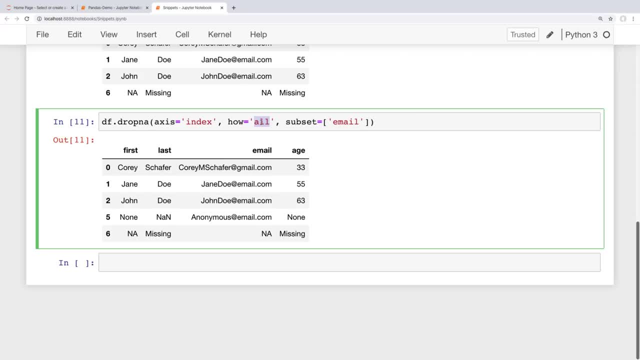 multiple columns to our subset. So what if we said, okay, well, in order for my data to be useful, I need either their last name or their email address, but I don't need both. So in order to do this, we could just say: okay, they need all of the. 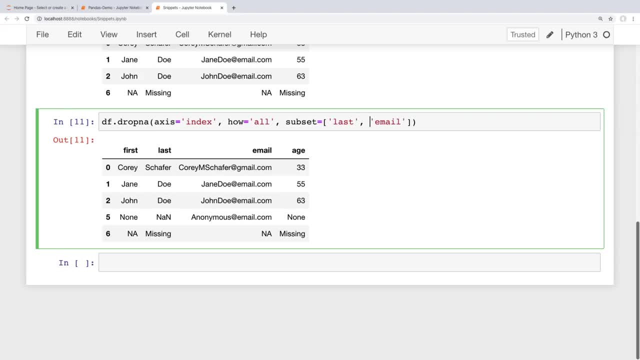 values in last name and an email or. I'm sorry there that I got that reversed. They don't need their last name and email. It just can't be that all of those values are missing. So as long as the last name or the email is there, then it shouldn't drop those rows. So if I run this, then we can see. 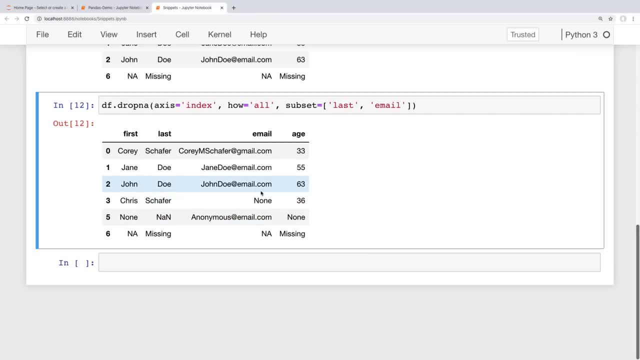 that we get some values that don't have an email but they did have a last name. And also we would get back some values that didn't have a last name but do have an email, just like the anonymous one here. It has an email but it doesn't have a last name. And again, that's because we 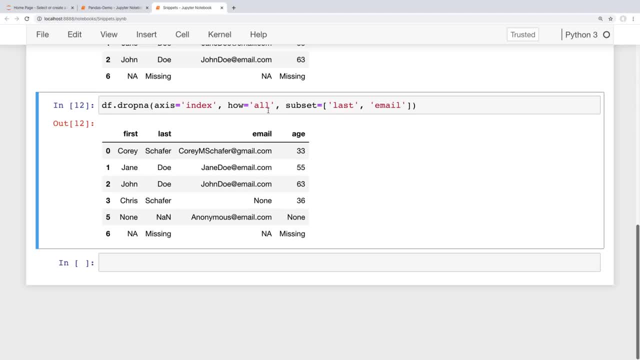 passed in all for our how argument, which means for a row to be dropped, both of the subset columns needed to be missing. Now, like we've seen in previous videos, this isn't permanently changing our data frame values. If we want to permanently change our data frame, then we'd have to add the. 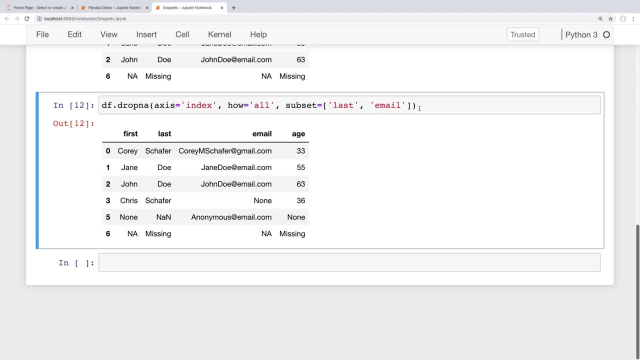 in place argument and set that equal to true here within this method. But we've seen that a bunch of times, So I don't think I'll go over that again here. Okay, so now let's get to these custom missing values. We can see down here that we have a row here that has some customized missing values. So 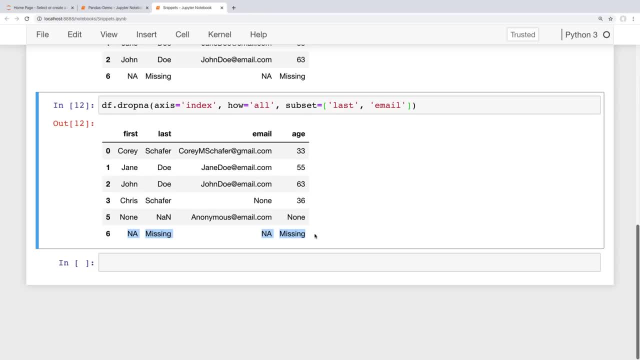 for example, maybe the people who got our data from didn't know what to do with missing values, So instead they just passed in a string of na, or they passed in, you know, a string of missing, like we have here. So how would we actually handle these? Well, it depends on how we load in our data. 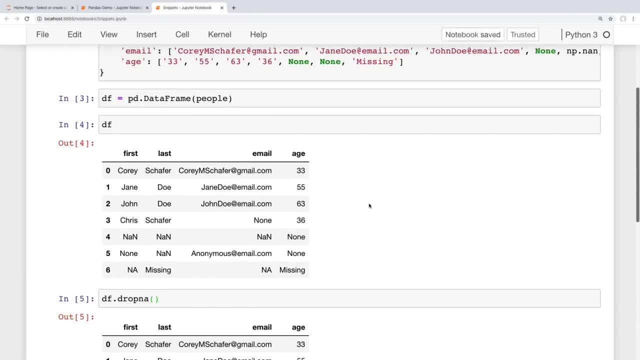 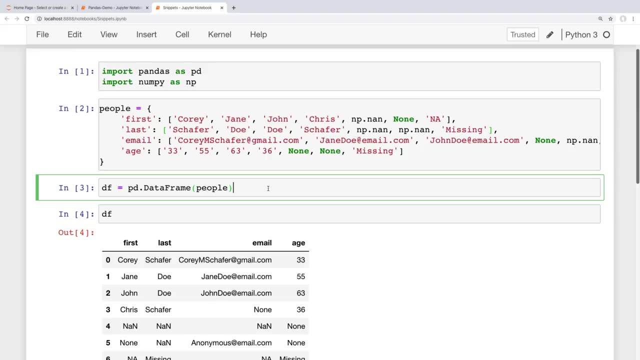 In this case, we've created our data frame from scratch by creating a dictionary and then creating our data frame here. So what we can do here is just simply replace those values with an na? n value. Now, if we instead loaded in our data from a CSV file, then we could do something different. But 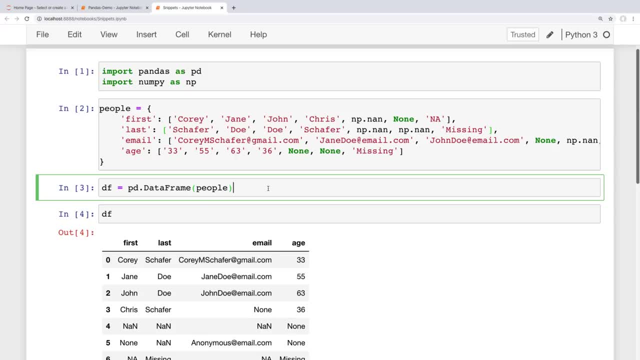 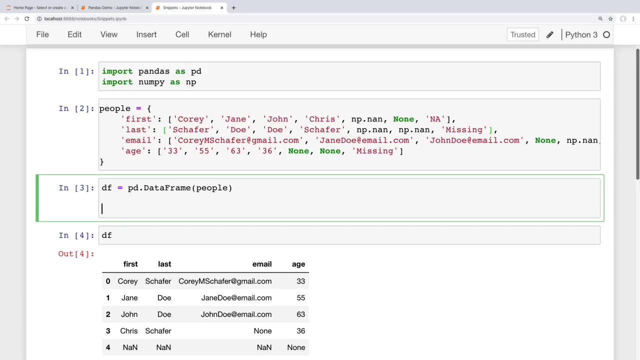 first I'll show this and then we'll take a look at the CSV file later, whenever I go over to the stack overflow data. So right here at the top, where we created our data frame, I'm going to use, with a proper numpy, na n value. So to do this, I'm just going to go a couple of lines down here. 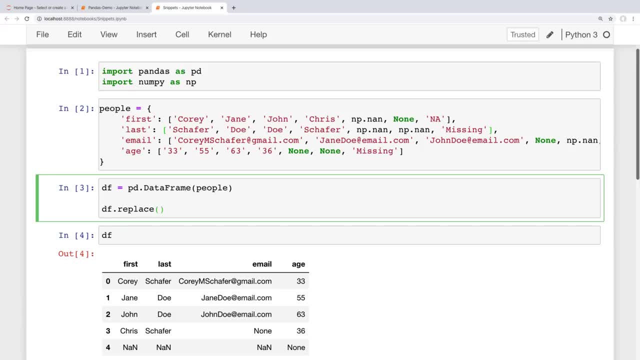 And we've seen this in previous videos. but we can use this replace here, And I'm replacing all the values in the entire data frame. So anytime we see a string of na, I'm going to replace that with numpy dot na, n, And again I am importing numpy up here as MP. So that's where I'm getting. I'm able. 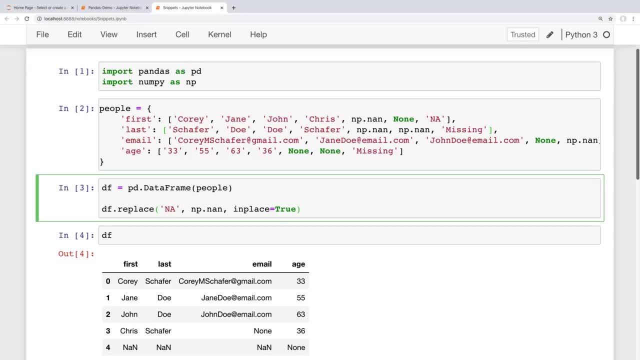 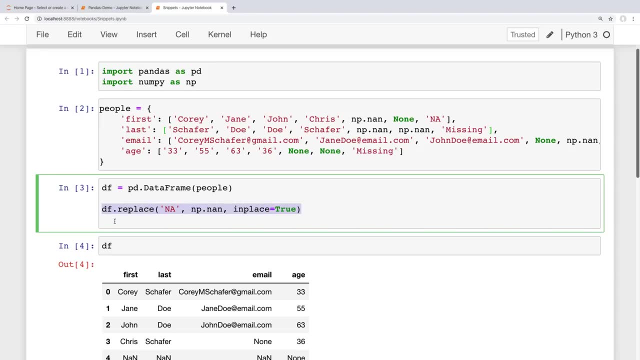 to modify that data frame. And then I want to say: in place, equal to true, because we actually want to modify that data frame. So if I run that, then that would replace those values. But I'm also going to replace this string of missing as well with MP dot na n values, And I want to do that in place. 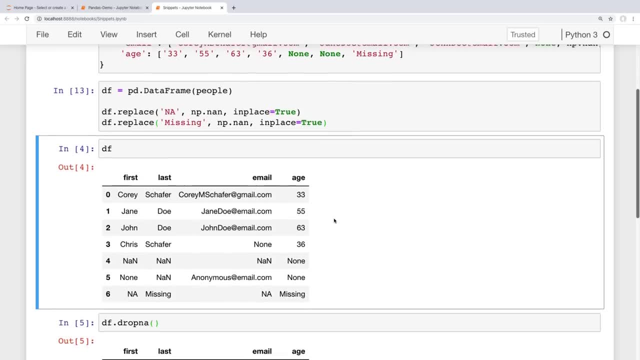 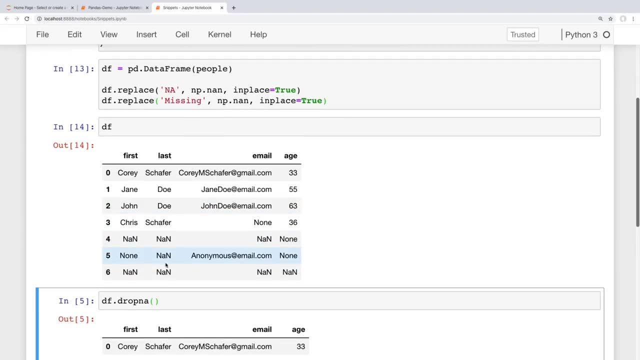 as well. So let's go ahead and run this. that should replace those values. And now, if I look at our data frame here, then we can see that we no longer have a string of missing values. So we can have that string of missing or na. These are now all na? n values. And now if we go back through and 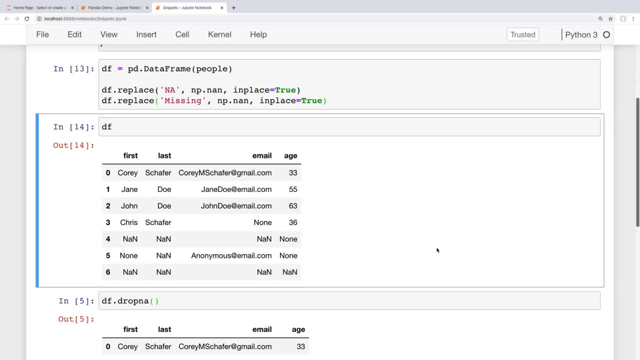 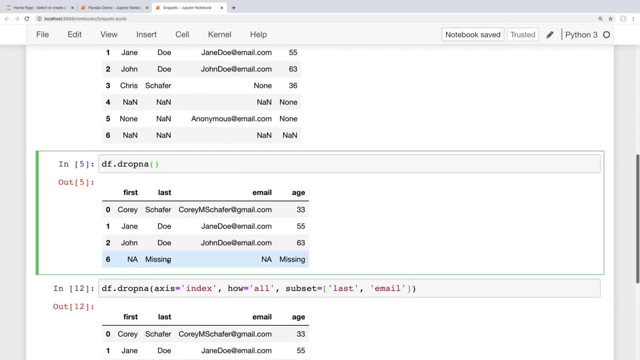 we run our cells where we dropped na values, then these custom values should have been replaced and it should treat those as missing values. So right here we can see what our previous result was, where we got this index of six with those custom values. If I rerun this now, we can see: 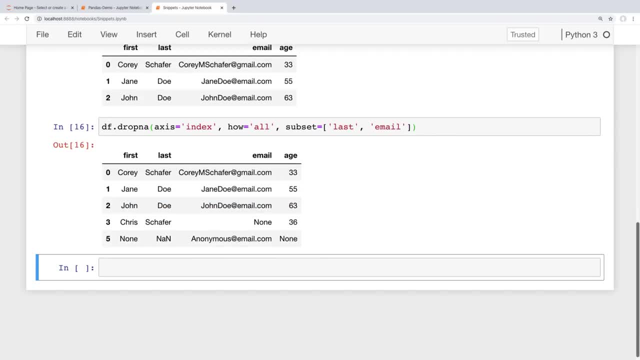 that. that's gone And the same with here. If I rerun this, then that is gone as well. Now, if you don't actually want to make any changes and we just want to see if certain values would or wouldn't be treated as na values, then we could just run the na or is in a method and get a mask. 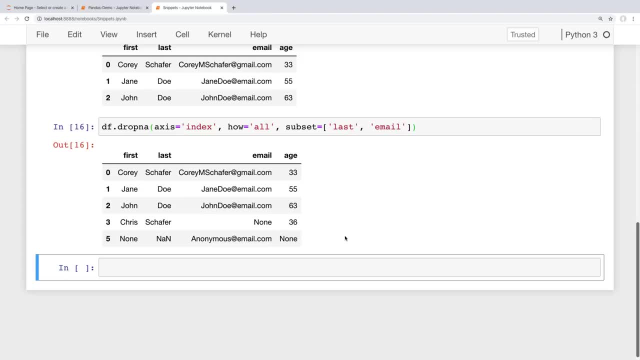 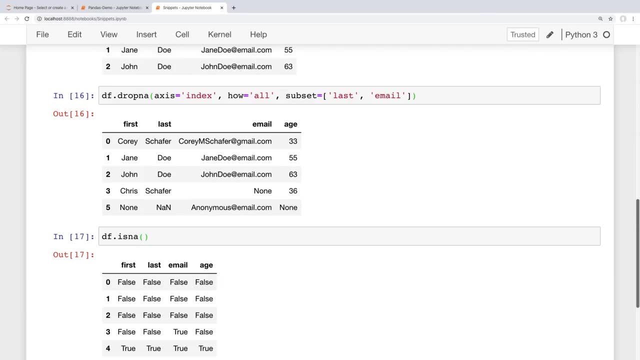 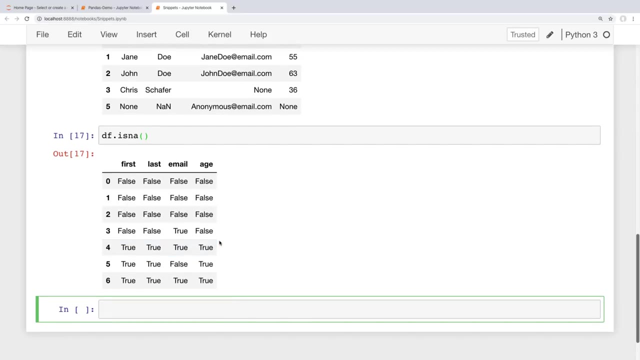 of values as to whether or not these classify as na or not. So let me just show you what I mean here. So I could say df dot is na, And this is just going to give us a mask here of values that are whether or not they are classified as an na value. So we can see that that's gone And then 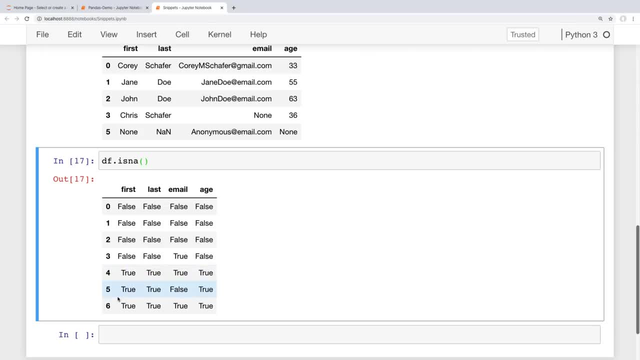 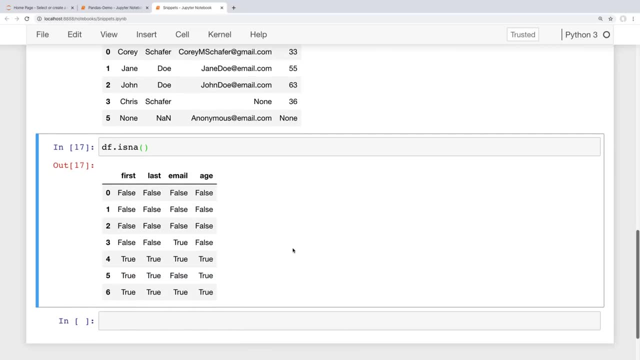 we can see that our row four here was all na values, And so same thing with our row six, And we can see some other missing values throughout here as well. Now, sometimes, especially when we're working with numerical data, we might want to fill our na values with a particular value. Now I'm 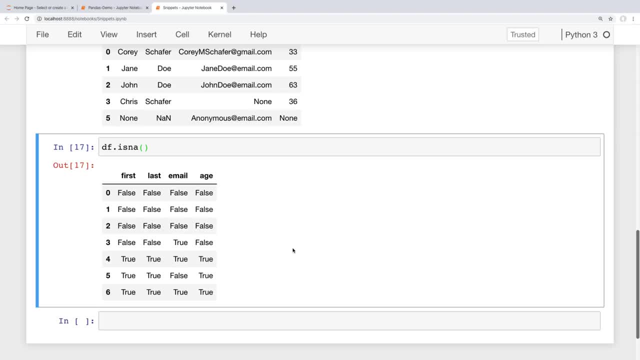 working with string data here, But sometimes it may might make sense to fill your na values with certain values with these as well. So, for example, let's assume that we were calculating grades for assignments or something like that, And you had some assignments that were in a. 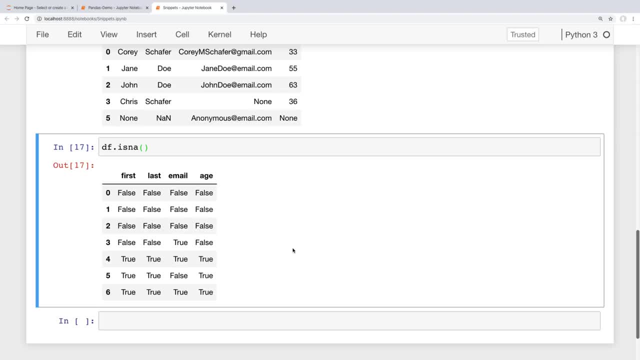 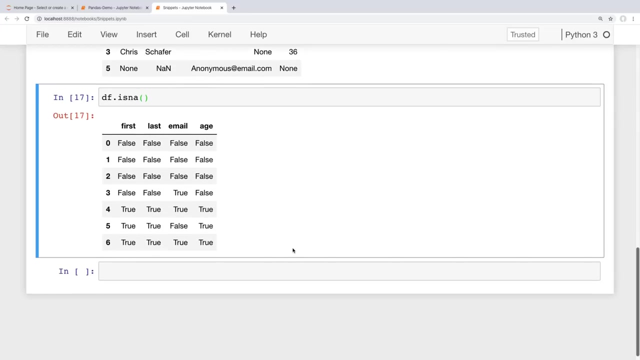 because the student never turned in the assignment. Well, at that point you could just decide if you wanted to score all missing assignments as zeros, so that you could probably calculate up the grades. So to do something like this we can use the fill in a method. So, for example, I could say: 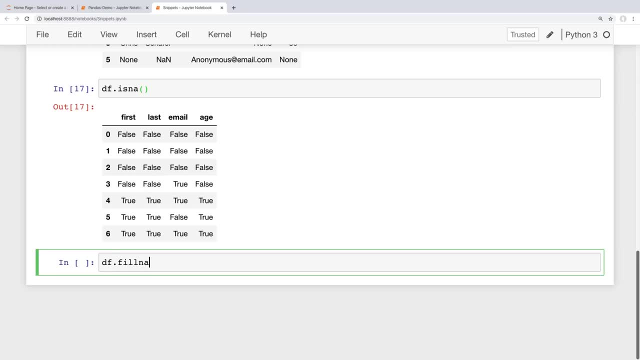 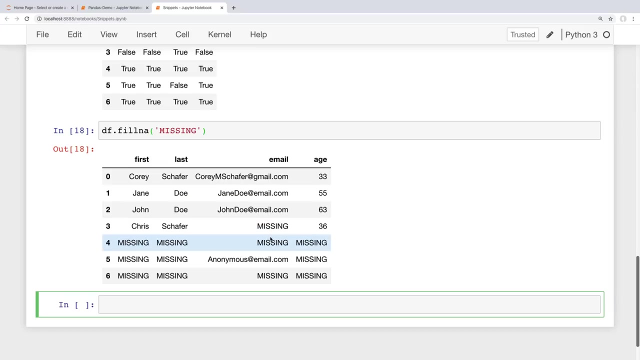 something like this: if I do a df dot, fill in a and then pass in a value. just to show you exactly what this is doing, I'm going to fill all of our missing values with this capitalized missing string here And if I run this then we can see that all of those missing or all of 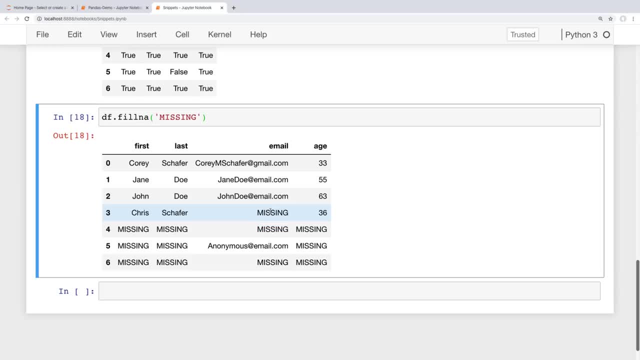 those na values were filled with this string capitalized as missing. Now, like I said before, I don't do this a lot with certain strings. I found this to be most useful for numerical data, depending on how you're doing your calculations. But you might want to fill in all of our missing values with this capitalized missing string here. 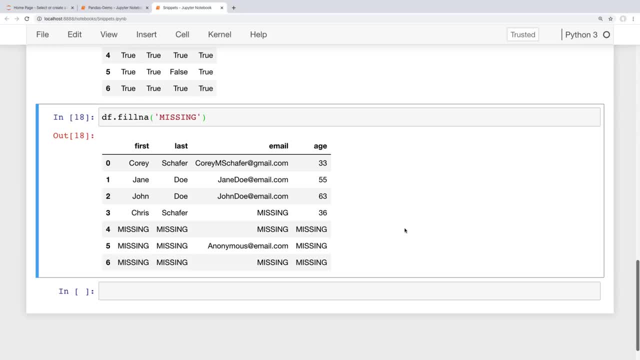 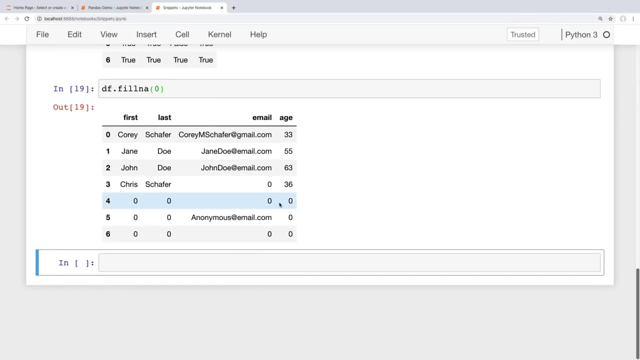 And if you want to give na values a value of zero or negative one or something like that. So if it would make sense with your data and you had numerical data to replace your missing values with a zero, then you could just run df dot, fill in a zero. And if I go ahead and run this, then we can see that that works on our data frame as well. And again, just like with our other methods, if you want those changes to your data frame to be permanent and carry over into other cells, then simply just add that in place argument and set that to true. 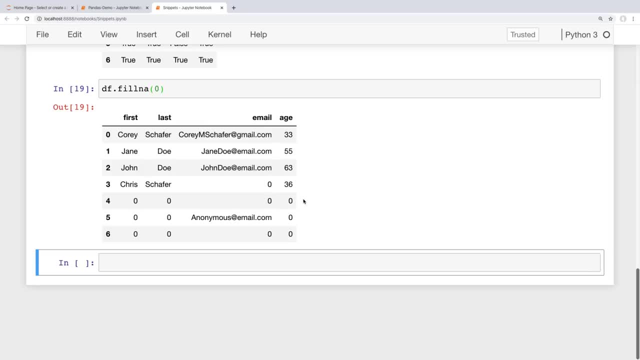 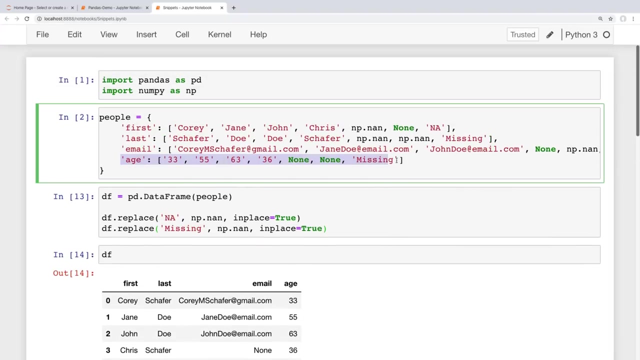 to make that change permanent. Okay, so now let's look at another common thing that we're likely going to need to do with a lot of our data, And that is casting data types. So I have another column in my snippets here that I didn't have in previous videos And I have up here. if we look, this is this age column. So let's say that we wanted to get the average age of all the people in this sample data frame. Well, right now, these might look like numbers when we print them out in our data frame down here, because 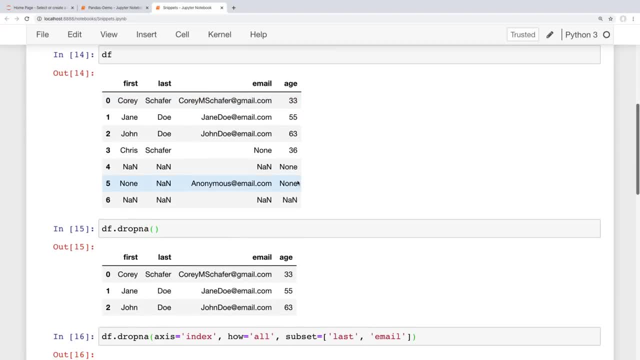 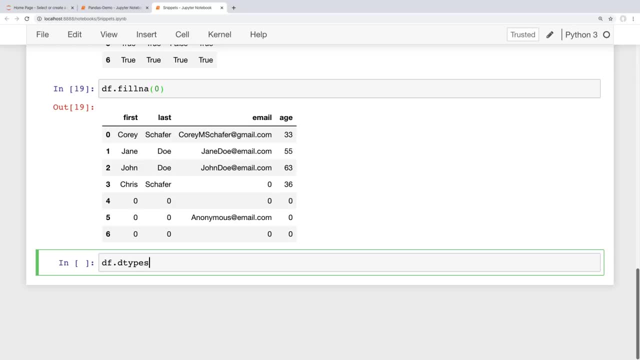 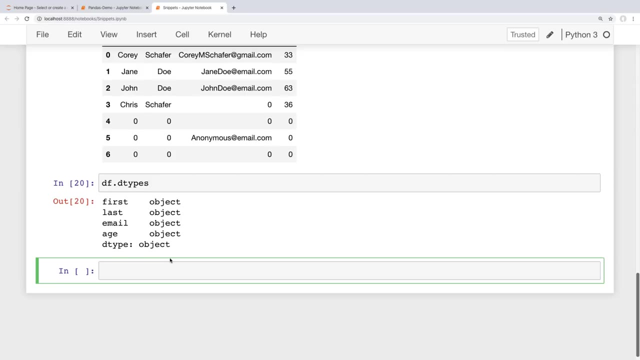 these are actually strings And we can see this if we look at our data frame data types. So to do this we can say df, dot, d types, And that's not a method, it's just an attribute. So if I run this here, then we can see that it says all of these columns are objects, And when it says it's an object, it likely means it's a string or a mix of different things. So in the latest version of Python or pandas- I'm sorry- they actually updated it so that there's actually a string data type. 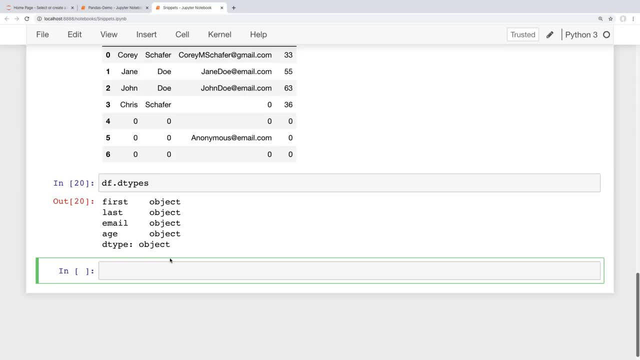 Now, but I'll do a video on those pandas version updates at the end of this series, since they actually released that updated version as I was writing this course. But don't worry, there's not a lot that's changed to where what you learn here will be outdated or anything like that. It's still mostly the same. But we can see here that our age column is a string because it's this object data type. So if we wanted the average age, then it wouldn't work as it is now. So 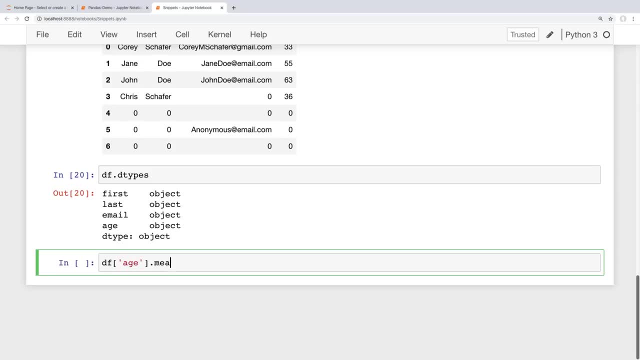 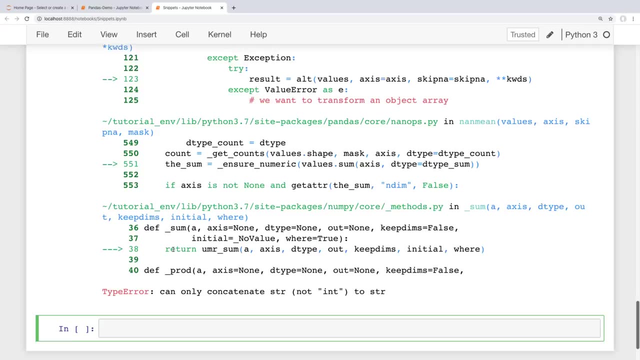 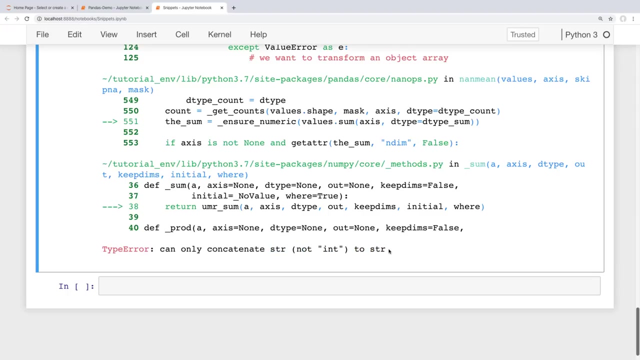 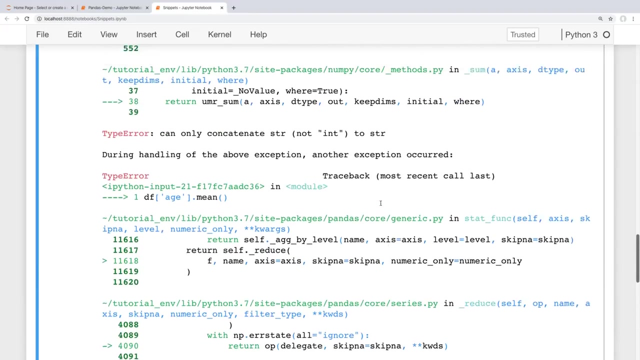 let's just see what this error looks like. So I'm going to grab the mean of that age column And if I run this then we can see that right now we get an error. And if I scroll down to see what this error was, it says: can only concatenate str, not int, to string. Now that might not be the most easy to understand error right there, But basically it's telling us that because that column is strings and not integers, So we need to convert that column to numbers instead of a string. 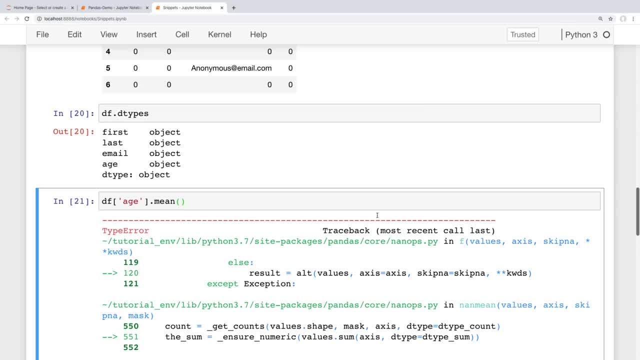 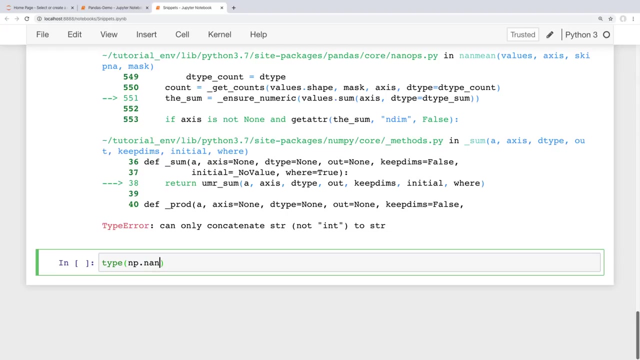 String. Now there's a caveat when doing this and this might throw some people off. So when we have in a in values in a column that we're trying to convert to numbers, then you need to use the float data type, And that's because the in a in value is actually a float under the hood. Let me go ahead and show this, just to show you what this looks like. So I'm going to look up the type of NP dot in a in And we can see that that is a float. So if we try to convert this column to numbers, 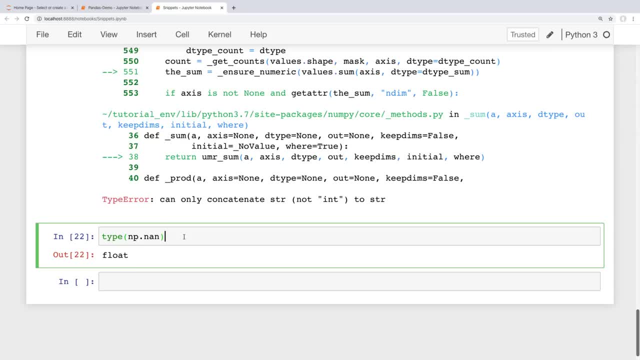 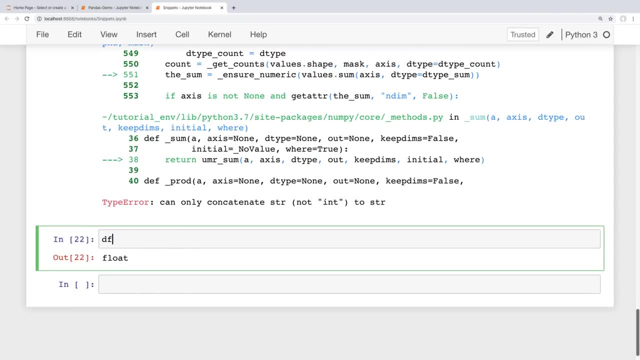 to integers, then it's going to throw an error when it runs into those nan values because it can't convert those. so if i was to say df and of age is equal to, and now let's try to convert these to integers. so the way that you cast data types here is we can just say: okay, i want the age column. 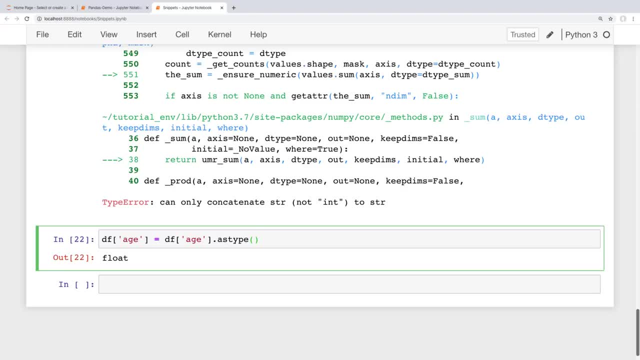 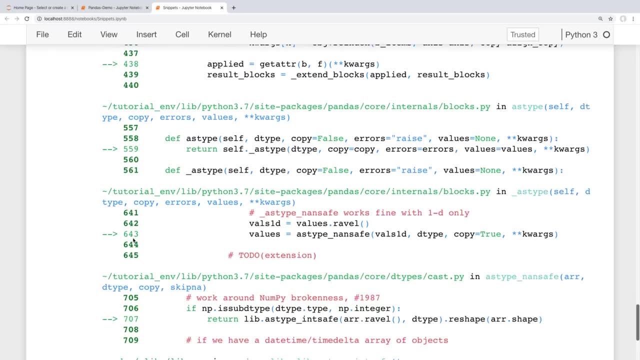 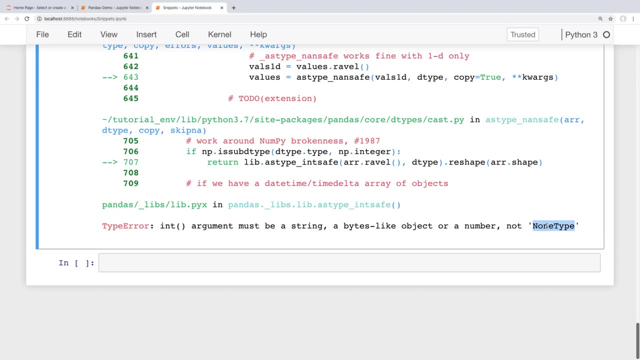 as type and now we want to pass in the type that we want. if i try to convert these to integers, then this is going to give us an error because we have some nan values, uh, so we can see here: int argument must be a string, uh, not none type. so when you're trying to convert these to numbers and 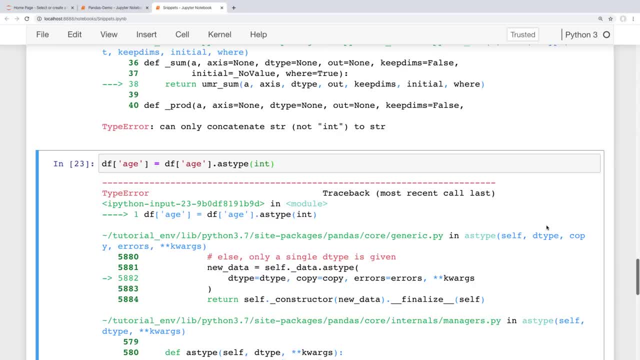 you have those nan values. you basically have two options here. if your column didn't have any missing values, then this would just work fine, we wouldn't even run into this error. but if it does have missing values, then you can either convert those missing values to something. 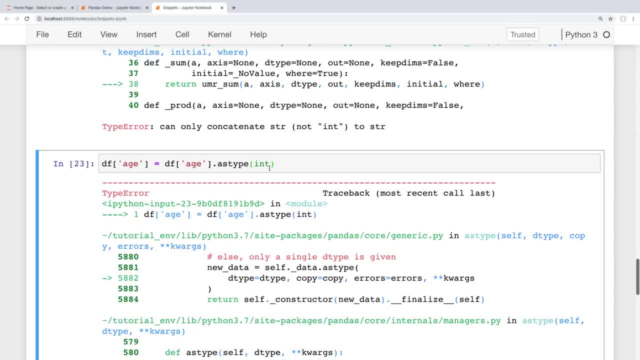 else like a zero, using the fill in a method that we saw before, or you can just cast that column to a float instead. now i think this would be a bad idea to convert those missing values to a zero or some other number, because we're trying to compute the average in this case, but depending 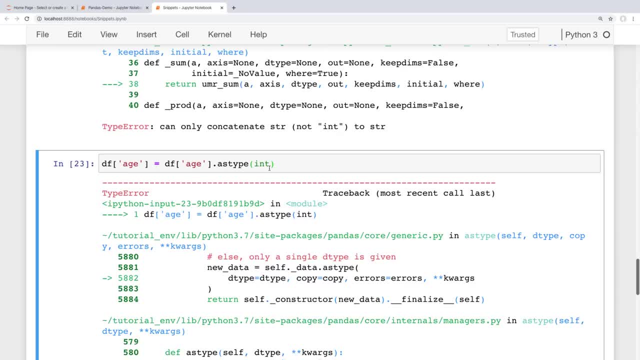 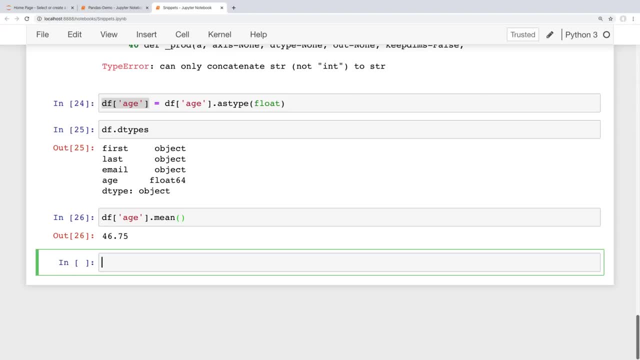 we don't want to do that, okay, so we've been looking at our small data set right now to test this stuff out. but now let's take what we learned here and learn how this applies to real world data and do some analysis on our stack overflow survey data. okay, so, first of all, i mentioned earlier that 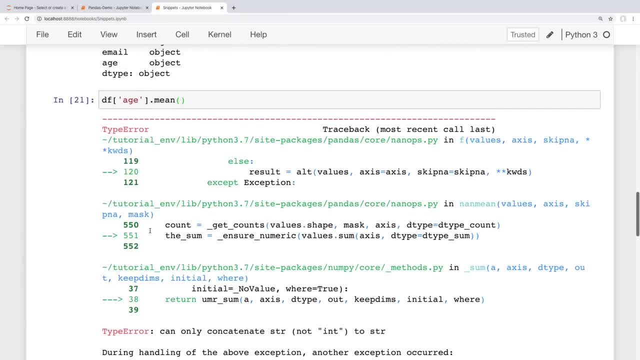 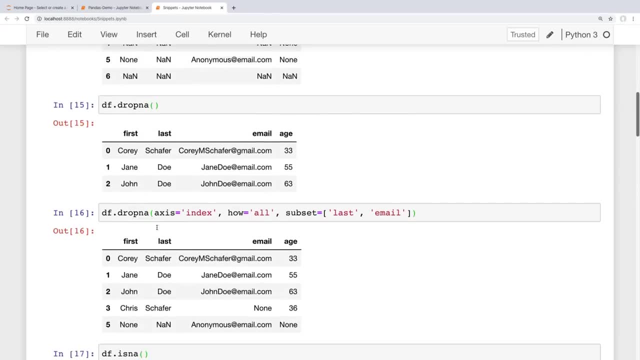 if we had custom values for missing data, then it's a little bit easier to handle these when loading in a csv. and what i'm talking about up here is up here at the top, where we replaced these custom values of the stack overflow data, and we're going to go ahead and just convert. 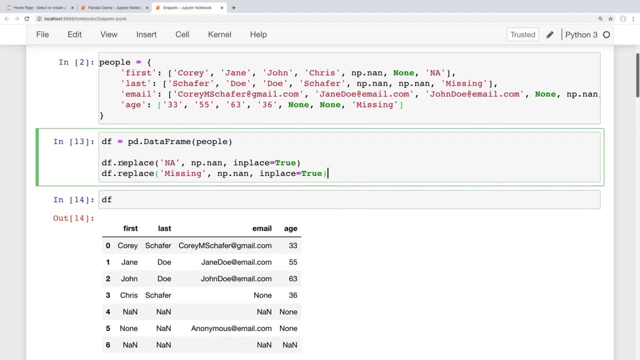 these to floats. so those nan values are going to be a number and i'm going to go ahead and just convert these to floats. so those nan values are going to go ahead and just convert missing values. let me show you how we would do this same thing, but loading in. 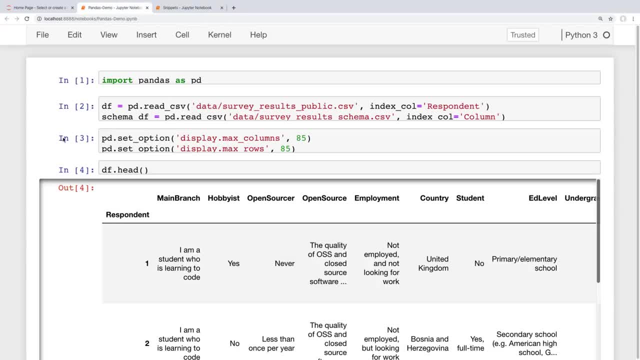 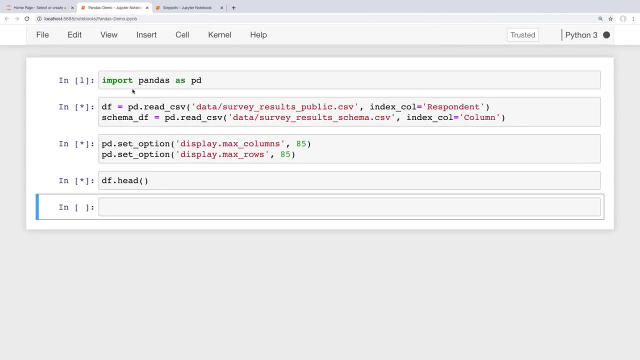 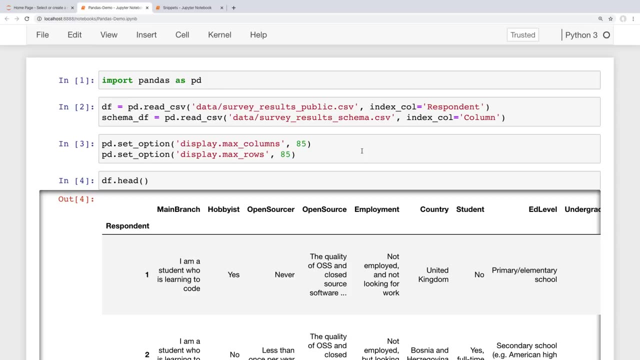 a CSV instead. so I'm going to switch over here to my stack overflow survey data. let me go ahead and rerun this, just to make sure that all of this stuff is running okay. so this notebook still running, that's good. and again, this is that stack overflow data that we would have been using throughout the series. 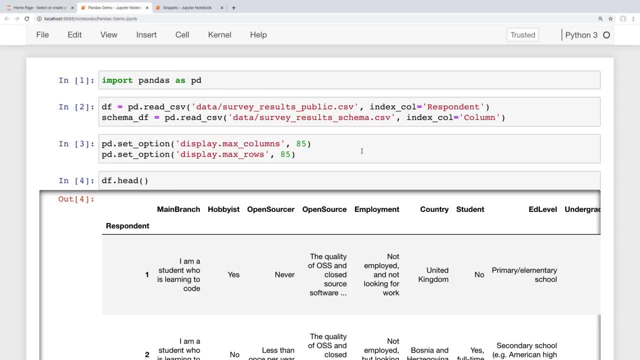 and if you'd like to follow along, then I do have a download link for this in the description section below. okay, so if I wanted to ignore those custom values when loading in a CSV, then we can simply pass in an argument of a list of values that we want to be treated as missing. so here's how we would do this if we had. 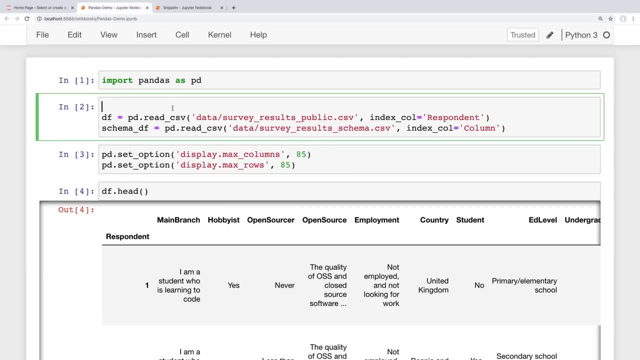 some custom missing values here in this CSV file, then I could simply create a list here of those missing values and I will just call this in a vows, and now I'll put in a list of values that we want to be treated as missing and I'll 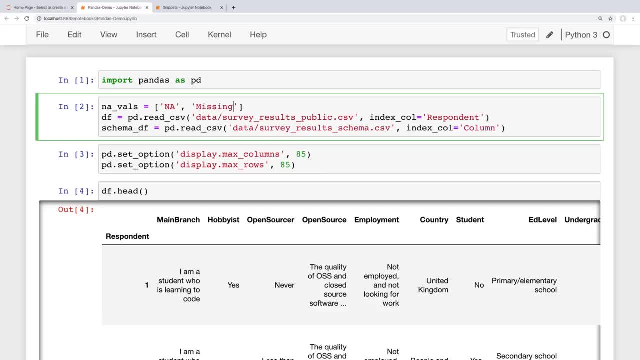 pass in a list of those. so let's say that we have some values that are a string of in a and a string of missing. so now what we could do here is just add in an argument and say: in a, values is equal to, and then that list that we just 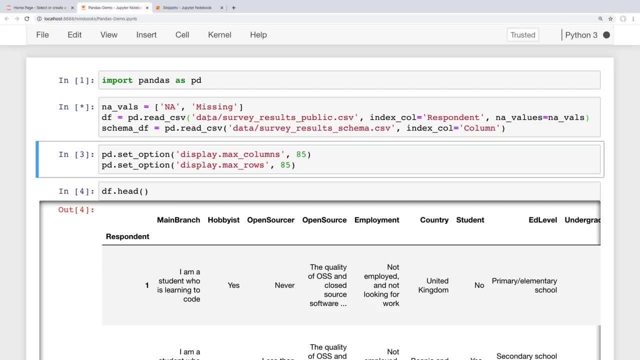 created and if we run that then we shouldn't get any errors. and when it reads in that CSV, then it will treat that list of values as missing values and give them an in a in result. so that's what I'm going to do here and I'm going to 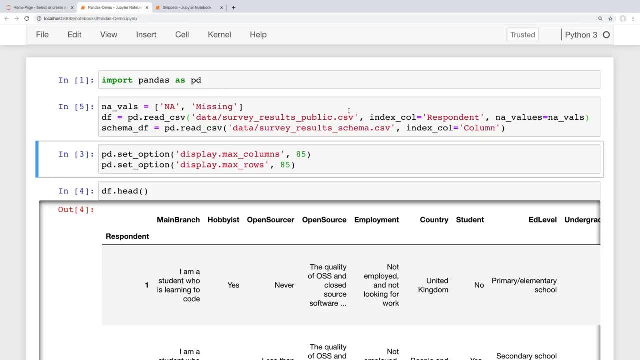 give that list an in result. so that's what I'm going to do here and I'm going to now. in this survey here, they did a good job of not having any weird occurrences like that, so that actually shouldn't change anything, okay. so now let's look. 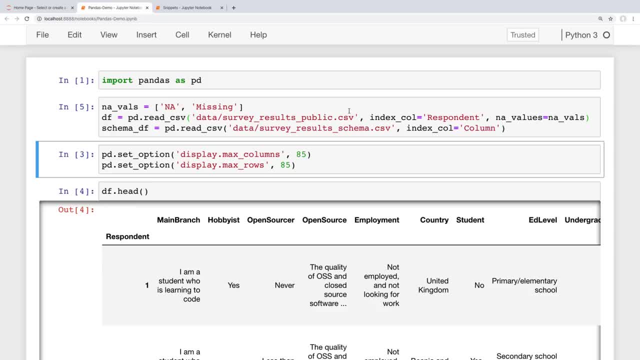 at an interesting problem with casting some values. so let's say that, for the developers who answered this survey, we wanted to calculate the average number of years of coding experience among all of them. now, that might be a good thing to know to compare your experience against the average. but let's look at. 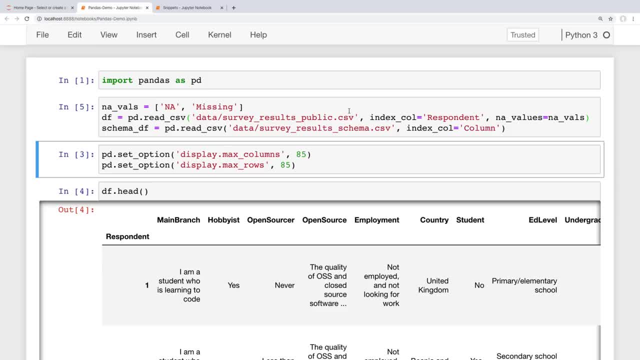 what this or why this might be some very difficult thing to do here, and the reason we did it is because it gives you the final answer that we can now run in this javascript and you'll be able to talk about all these parts in just a be difficult to calculate with this data set And us calculating this solution is actually going to. 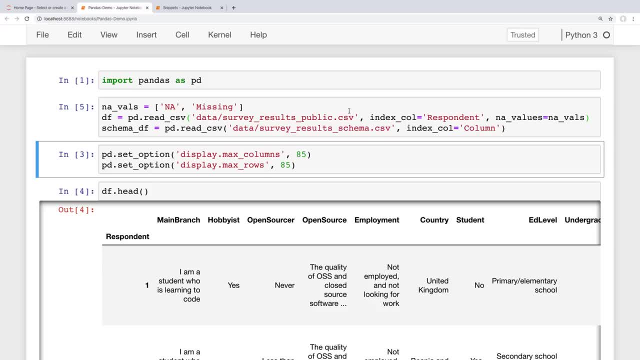 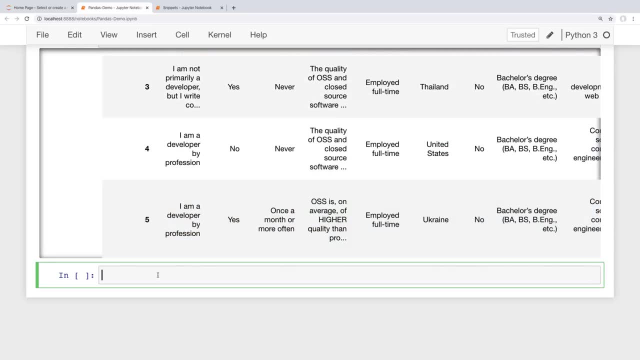 apply several concepts that we've learned so far throughout this series. So the column to view the answer for this question in the survey is called year's code. So let's look at some of these answers. So I'm just going to look at the top 10 answers for year's code, So I will do a dot head. 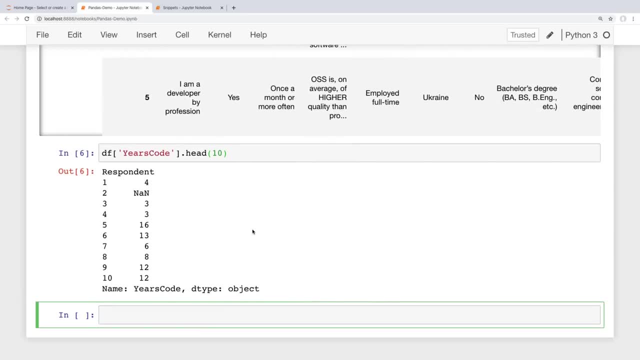 and let's look at the top 10.. So if I run this, then at first glance this doesn't really look like it'll be a problem. We just have a bunch of integers and the number of years that different respondents have been coding, So you might think that we can just grab the mean of this column. 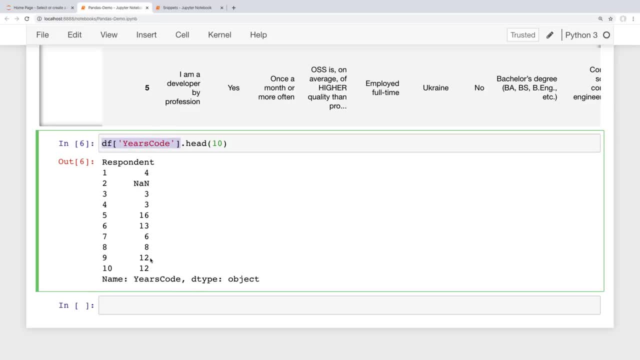 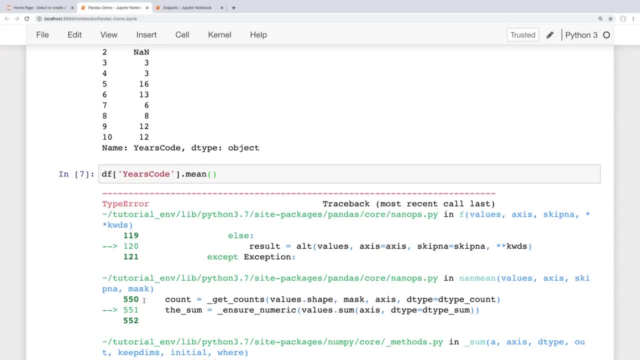 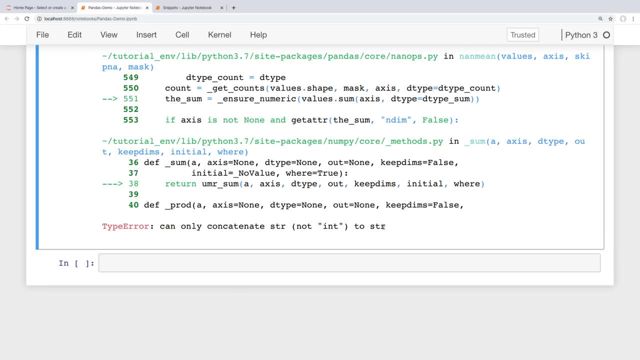 simply by saying, okay, if we just have a bunch of integers here and some NAN values, that's fine, Let's just grab the mean of that column. But if I run this then we get an error. And if I down here then it says: can only concatenate string to string. And we saw the same error in: 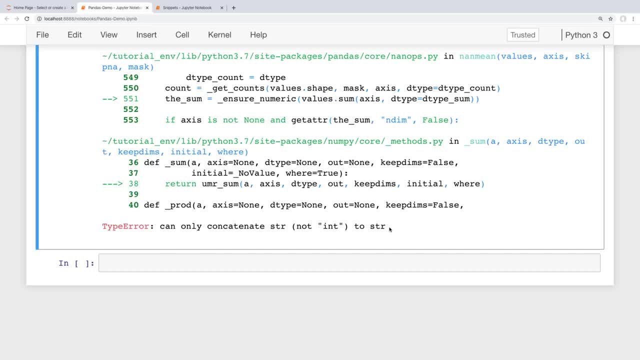 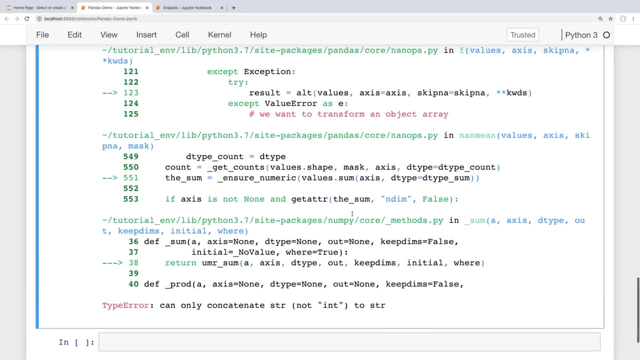 our smaller data set, where the column was actually being loaded in as a string instead of numerical data, And we should know how to handle this by now, since we did it in the smaller data set. So let's try that. So let's try to convert this to floats and then take the average. So let me go. 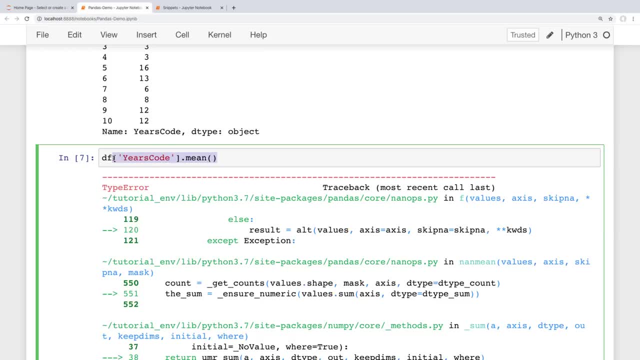 back up here to the top, where we ran this And instead of running the mean here, I'm going to say, okay, well, let's convert this to a float so that we can grab that average. So I will say as type: 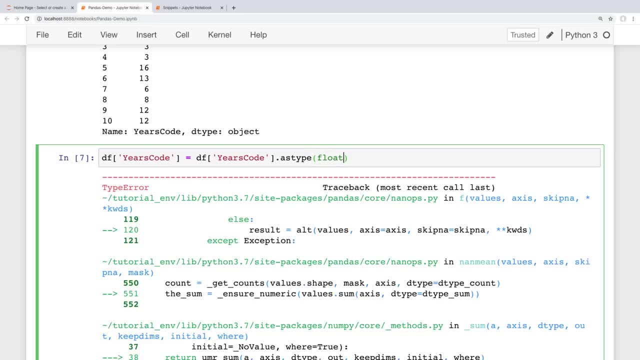 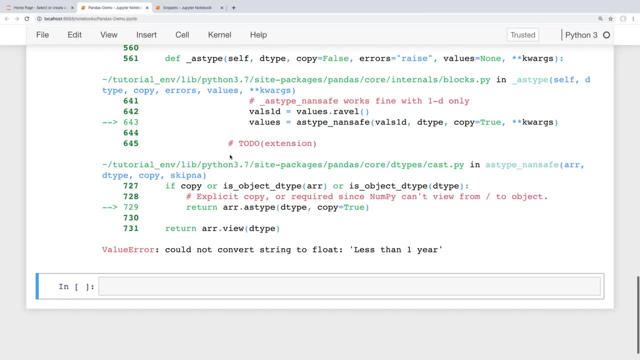 and we want to convert this to a float since there are in a in values. So if I run this then we still get an error. So we didn't get an error in our smaller data set here. So if I scroll down then it says: could not convert string to float And the string that 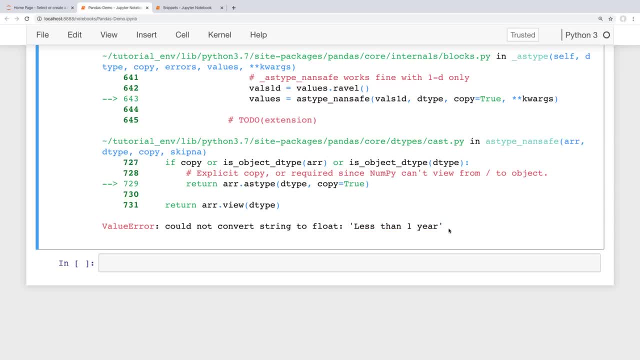 it couldn't convert was less than one year, So this might be something that we didn't expect here. So obviously we don't just have numbers and NAN values in this column. There is actually a string value that respondents could select that is equal to the string of less than one year, for 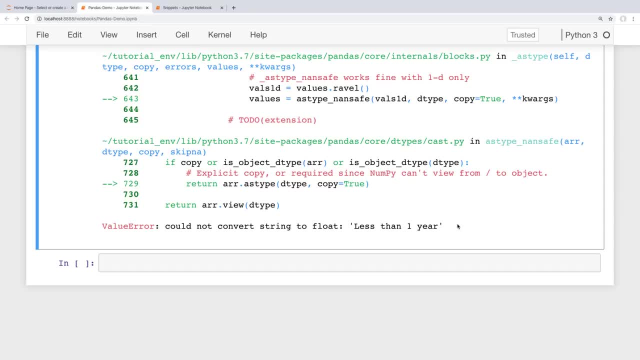 coding experience. So let's look at all the unique values of this column so that we can see exactly what's in here, in case there are more strings like this- And I don't believe we've actually seen this in the series yet, Maybe we have, I can't really remember- But if we want to view, 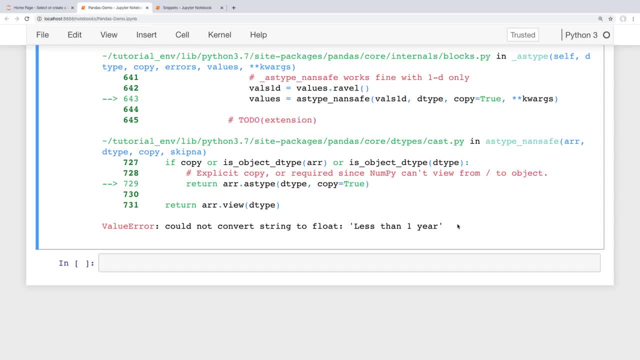 unique values of a series, then we can simply use the unique method. So we could also use the value counts method that we've seen several times before. if we want to count all the unique values, But we don't really want to count them, We just want to see all the unique values in this column. So to do: 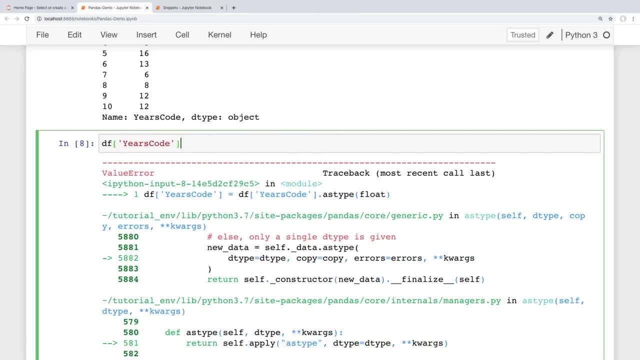 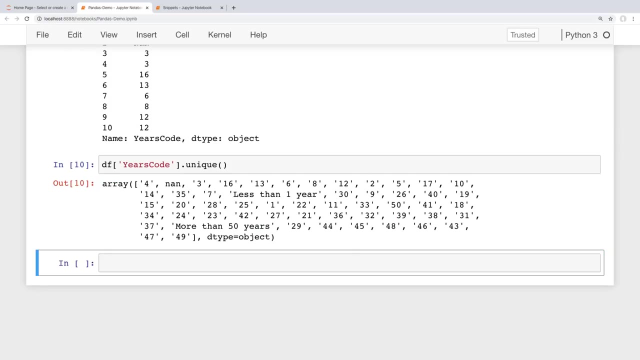 this. I'm going to say df and then access that year's code column unique: unique. That is a method. So if I run this- whoops, and I spelled this wrong, Sorry, having a hard time typing today. Okay, so if I run, 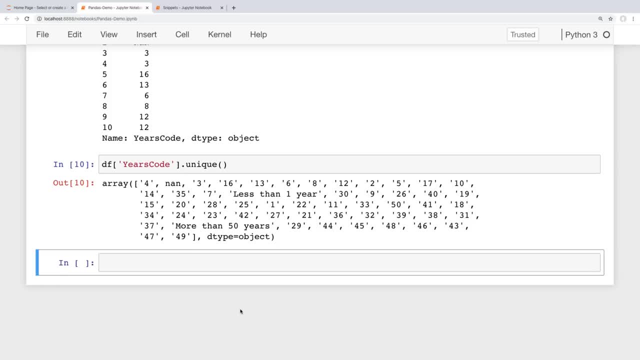 this, then this gives us all the unique values of that column And, as we'd expect, there are a lot of numbers, But we see that we also have some strings that are mixed throughout these numbers. Now we also have NaN values here, but we're not going to worry about those. We just want to ignore the NaN values. 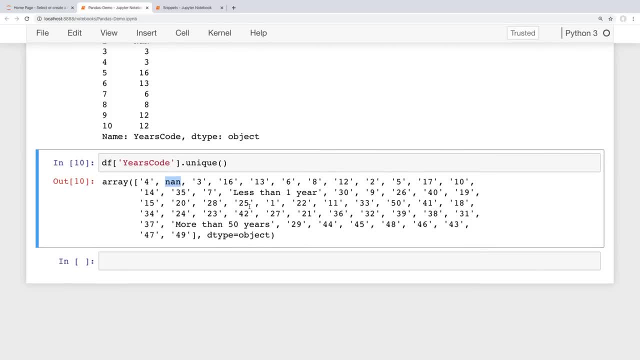 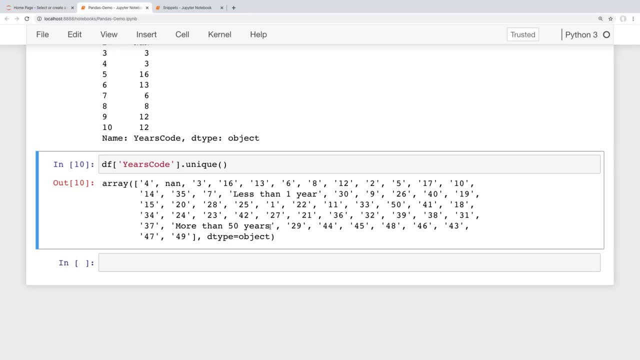 because that's just people who didn't answer the question, But we can see that the strings that we have throughout here are less than one year and more than 50 years of coding experience. Okay, so those are our only string values, So I'm going to replace those with numbers so that we can get. 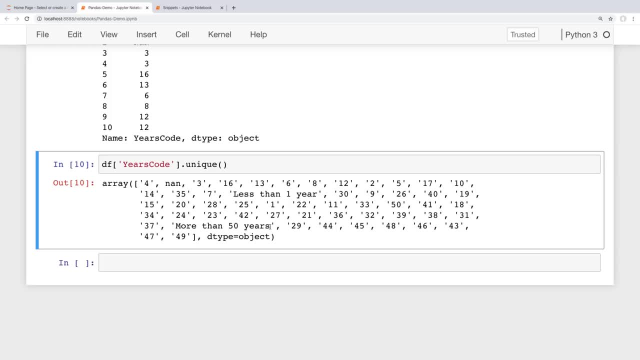 an idea of the average years people have been coding. So let's go ahead and replace less than than one year here with a zero, since that's basically the same thing: if somebody's been coding for less than a year, then they've been coding for basically zero years. so to do this. 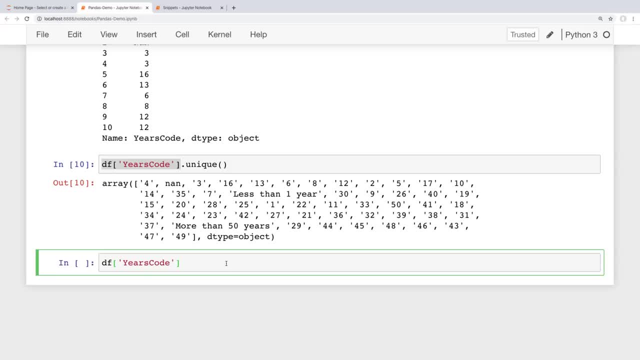 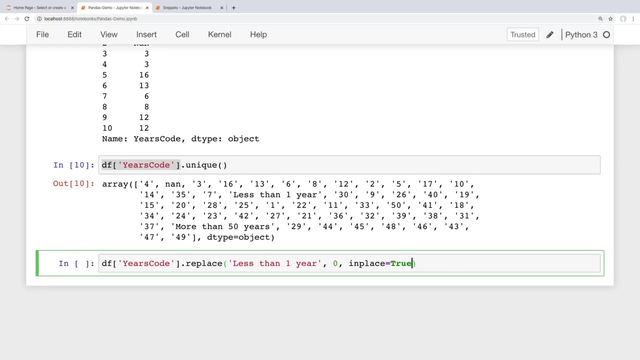 I can say DF dot years code and access that column and then we can just replace that value of less than one year and let's replace that with a zero, and we also want these to be in place equal to true, because we actually want to modify that data frame. so if I run that, 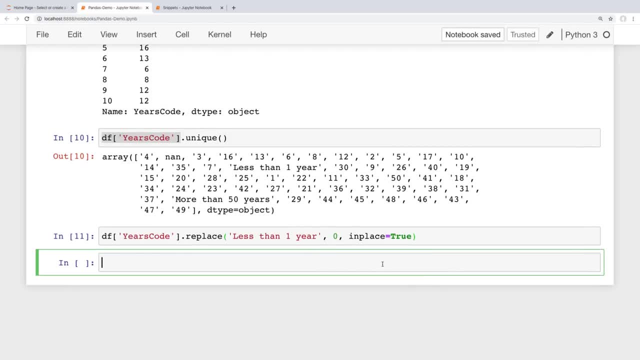 then it should make that replacement, and now I'm also going to replace the value for more than 50 years here, and this is going to skew our results a bit, depending on how we want to do this. I'm simply going to replace this with the value of 51. 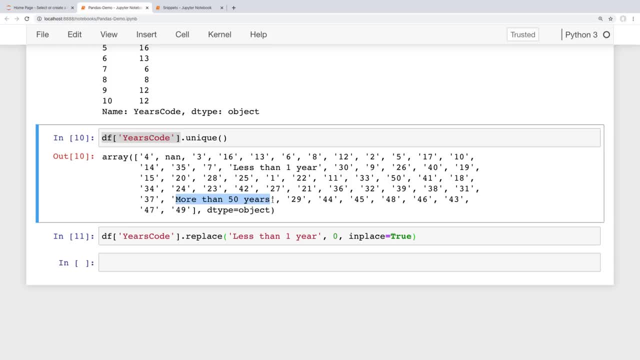 there may be some people who have several more, more years of coding experience than 51 years, but I can't imagine that would be that many people who have, you know, coded many years greater than 50. so i'm just going to fill this in with 51. 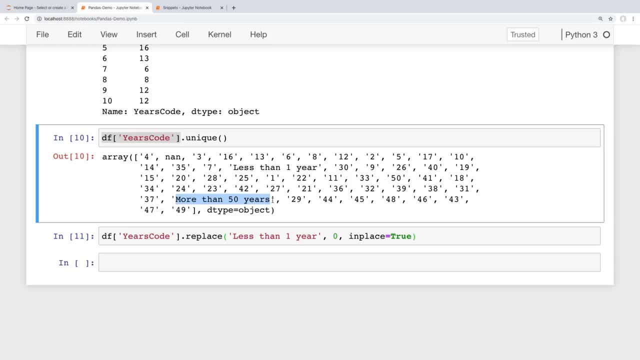 but, like I said, depending on what we pick here, it could affect our results slightly, but not by a lot in this case. so I'm just going to grab the same replace value here and instead I want to replace more than 50 years, and I'm going to replace that with a value of 51. so now let me 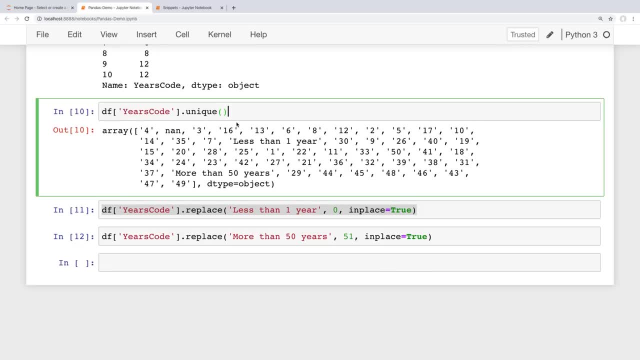 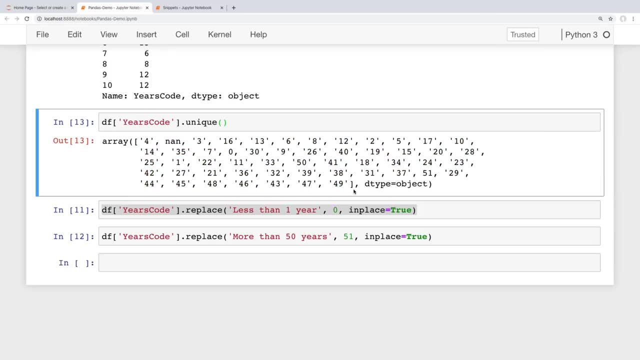 go ahead and run this, and if we want to look at these unique values again, then we could look at these. and now it doesn't look like we have any strings in here, but we can see here that this is still a d type of object, which means that it's not actually reading this in as floats. so if we scroll, 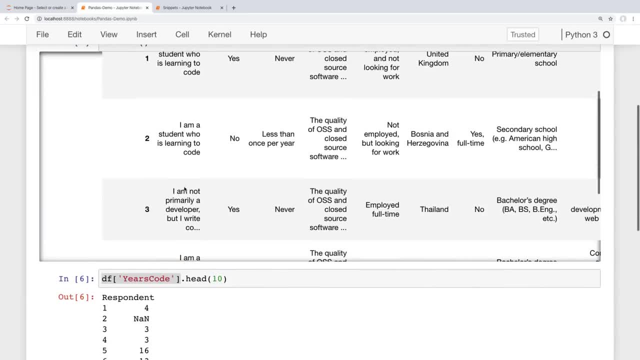 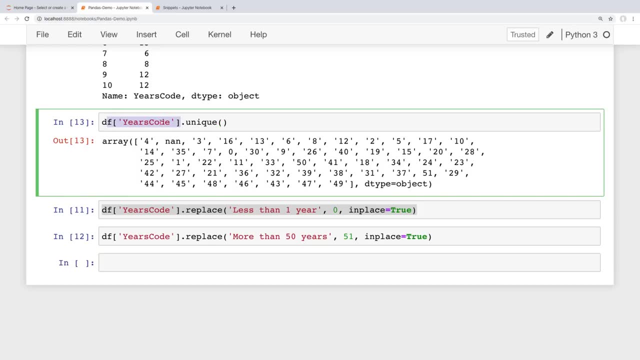 back up here a bit. oh, actually, i think i um overwrote that line. yes, i did so. let's just try that again. so what i want to do here is i want to convert this to a float, and this is what uh gave us an error before because we had these strings in here and it didn't know how to convert these. 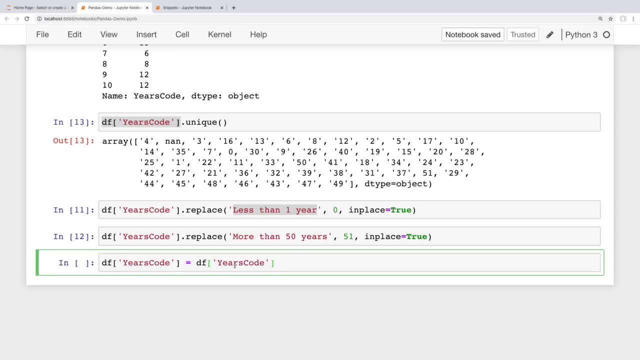 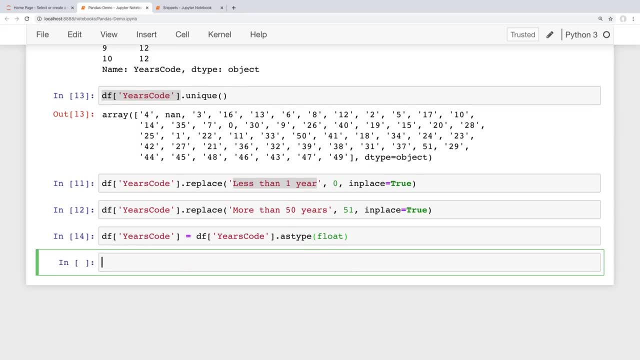 to a float. but now we should just be able to see: say: okay, i want to convert that as type set that to a float, so let's run that. and we didn't get an error this time, so that's good. and now we should be able to view the average numbers of. 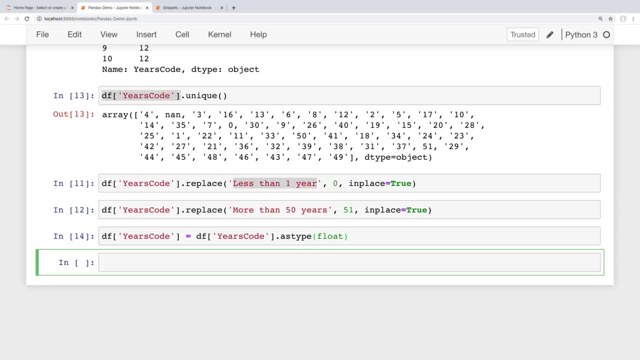 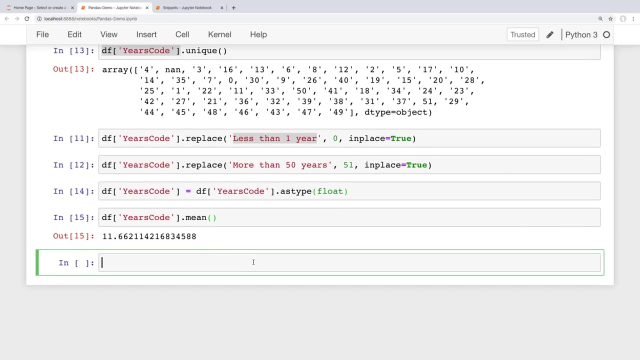 or average number of years of coding experience of the developers who filled out this survey. so to do this, I'm just going to say, okay, DEF, data frame access that column, grab the mean of that column. so if I run this, then we can see that now we get that average back. so the average that we got here was about eleven and a. 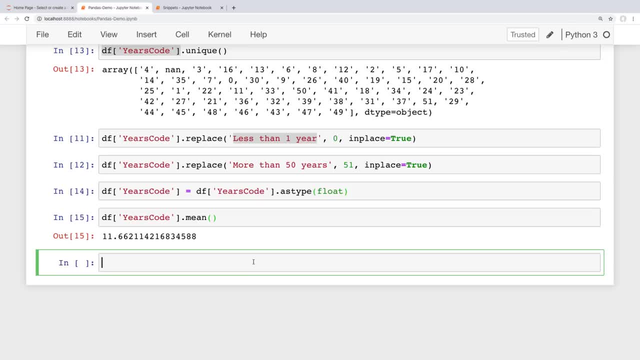 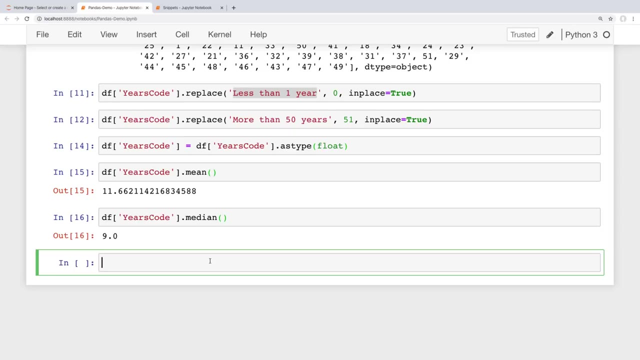 half years of coding experience as the average years for developers who answered this survey, and now you can do other analysis on this as well. so, for example, if we wanted to see the median, then I could run that, and the median comes back as nine years of coding experience. so hopefully that real-world. 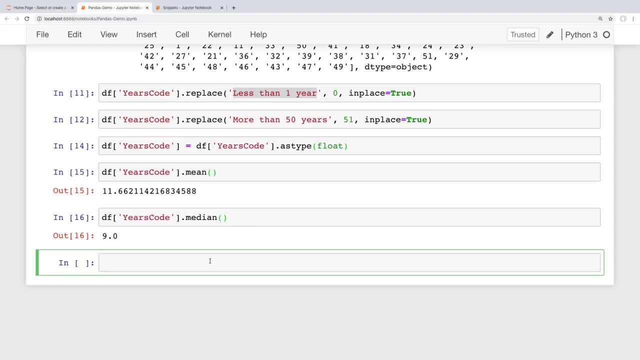 example, helped explain why it's important to know how to cast these values and understand what's going on there. there's always going to be data that is messy or not in the format that we want it in, so knowing how to handle these missing values and cast these values to different data types is really 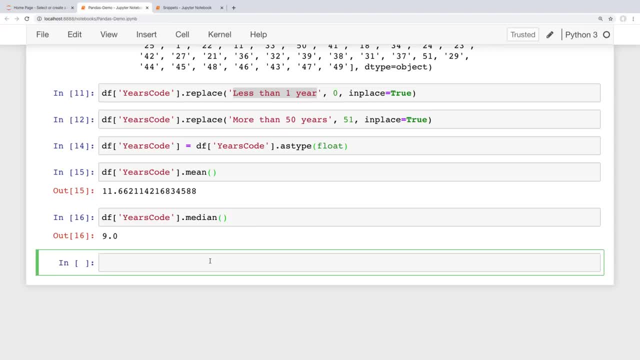 going to be essential when working with pandas. okay, so before we end here, I'd like to thank the sponsor of this video and mention why I really enjoy their tutorials and that is brilliant. so in this series, we've been learning about pandas and how to analyze data, and Python and Brougham would be an. 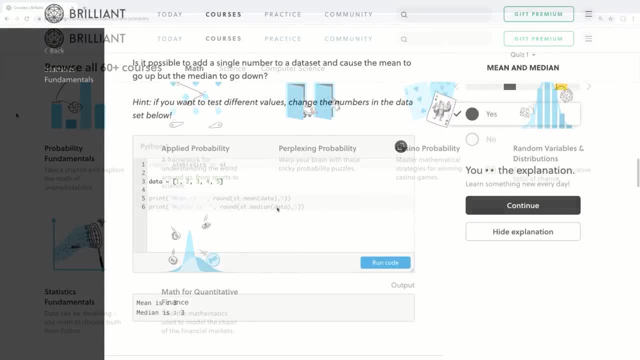 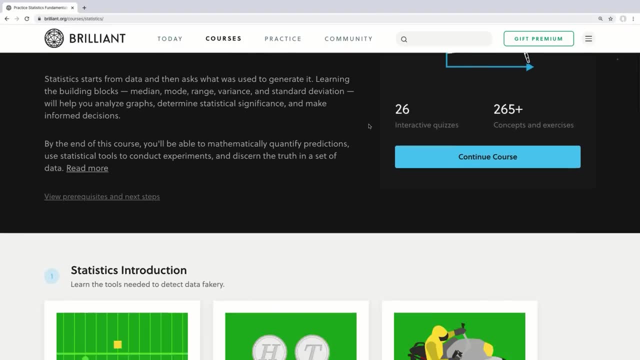 excellent way to supplement what you learn here with their hands-on courses. they have some excellent courses and lessons that do a deep dive on how to think about and analyze data correctly. for data analysis fundamentals, I would really recommend checking out their statistics, Emmim, which shows you how to analyze graphs. 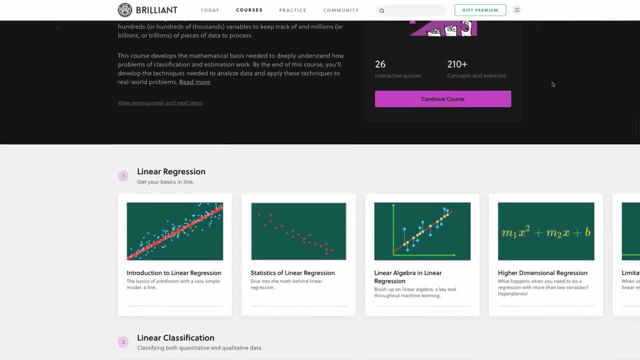 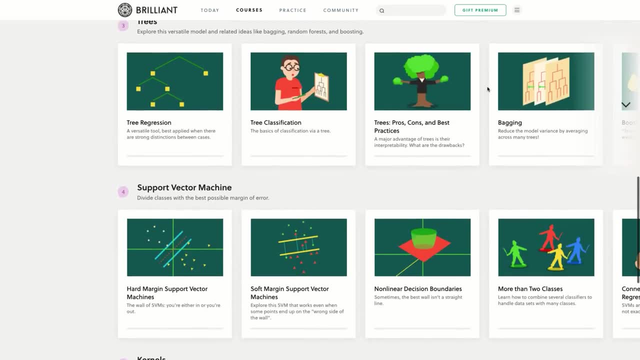 and determine significance in the data, And I would also recommend their machine learning course, which takes data analysis to a new level, where you'll learn about the techniques being used that allow machines to make decisions where there's just too many variables for a human to consider. 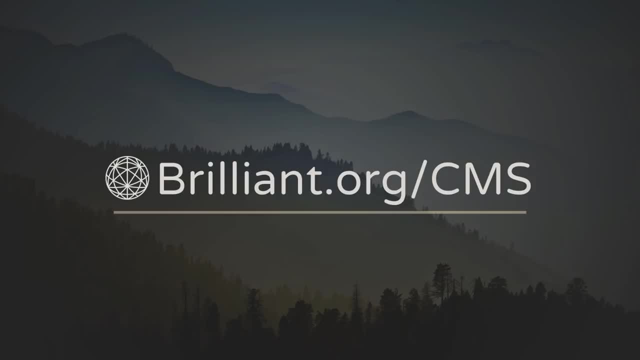 So to support my channel and learn more about Brilliant, you can go to brilliantorg forward slash CMS to sign up for free And also the first 200 people that go to that link will get 20% off the annual premium subscription And you can find that link. 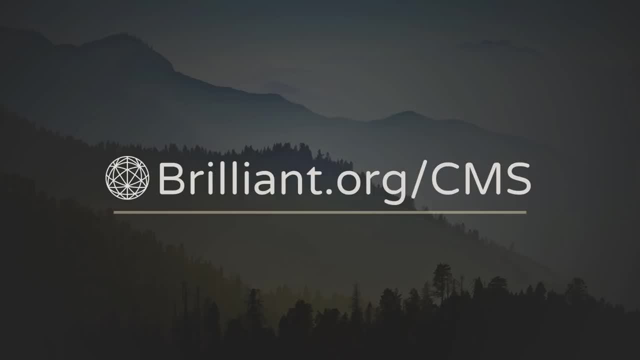 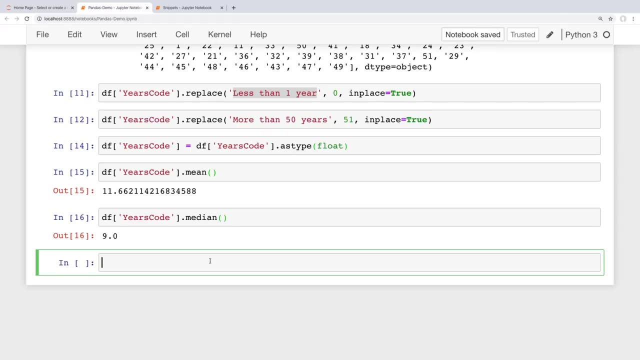 in the description section below. Again, that's brilliantorg forward slash CMS. Okay, so I think that's gonna do it for this Pandas video. I hope you feel like you got a good idea for how to handle these missing values and cast our data to different data types. 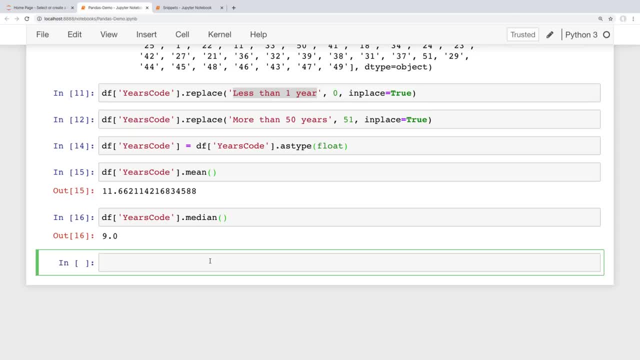 so that we can do exactly what we wanna do in terms of analyzing our data. Now, in the next video, we're gonna be learning how to work with dates and time series data. Now I've been using the Stack Overflow survey data for this entire series.